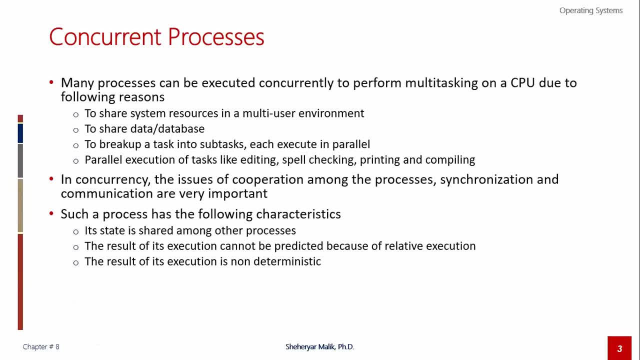 competing with each other to share the CPU. but then I'm very important is to share the data, the database, so they are working on. or then there can be content processes- just some net reading about the TV. divide the task into subtasks so that they can execute in. 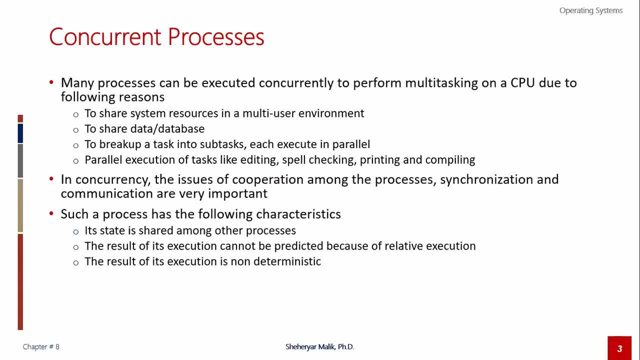 parallel. so they are content processes because eventually they are going to achieve the total in naturally the objective to execute that process. and then again we can have a parallel execution of tasks within one process which are actually doing multiple or different types of tasks, but eventually again they are contributing to the same. for, for example, word processor just. 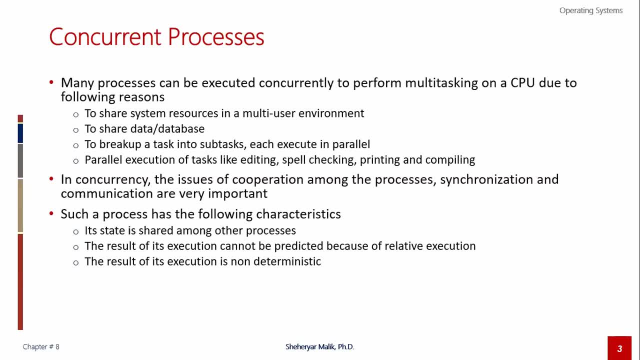 from our ahead. those can. there we would be doing an editing, formatting, file checking, printing or other stuff together in one. so these are called concurrent processes and the one of the major issue is that is operation, because cooperation among the processes is really really very insistent. so job cooperation, Hoga. so 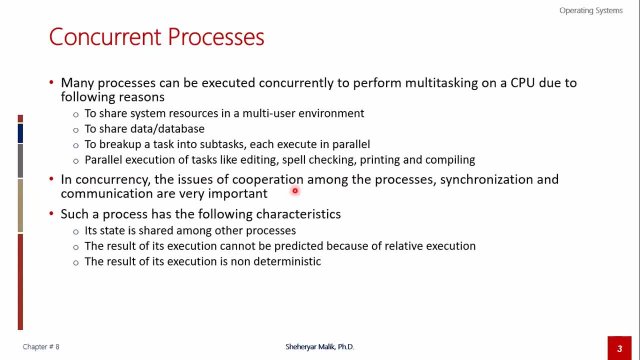 just you cooperate, cutting getting need to synchronize. synchronization of each like schedule, care in which order they are going to execute or they are going to access the shared, in which order we will execute, in which order we will use these things. That is the synchronization and once they, 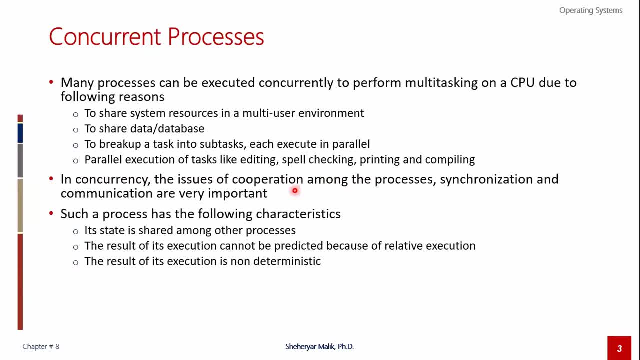 have to do the synchronization and the cooperation. they need to have a very effective communication among them. Their communication between them should be very effective. When we talk about concurrent processes and we say that, yes, they need to synchronize with each other, they have to communicate with each other. they have to 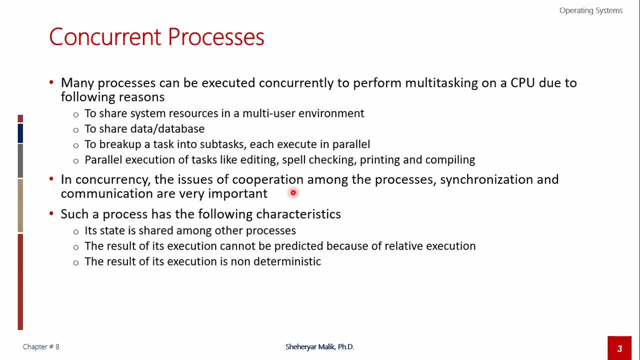 cooperate. so they need to have some certain characteristics, some qualities or characteristics which they need. Number one, very important, is that their state needs to be shared among the other processes. So the current process, the concurrent processes, its state is shared among other processes. 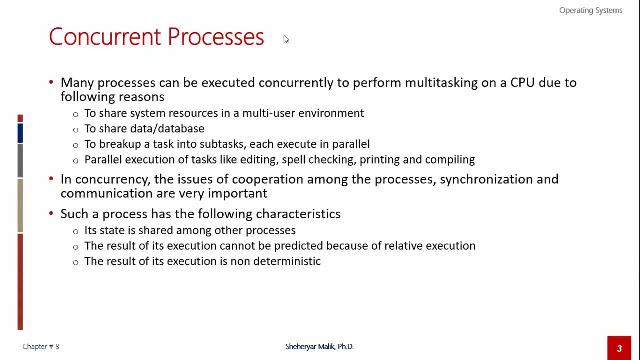 Second, very important, is that results of execution cannot be predicted because of violated execution, because the sharing of the data, the results of the execution, it's not deterministic. so because it's it's not deterministic. so because it's not deterministic, So it's not deterministic, So it's not deterministic. 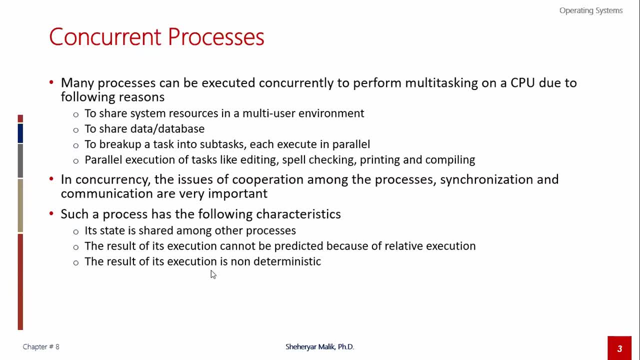 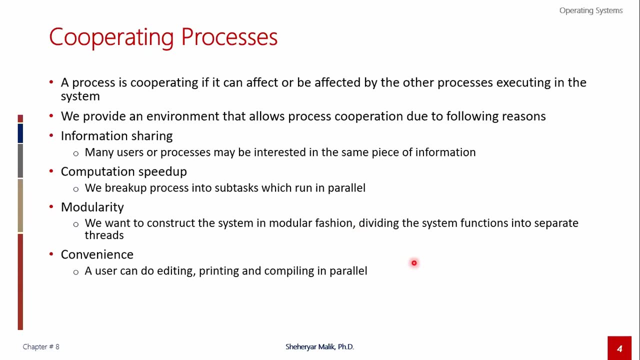 you cannot predict it, so that's why it's also non-deterministic as well. so cooperating processes as a processes which affects other processes, or they can get affected by other processes, or generally, we provide the cooperation mechanism in our systems. one of the reason is information share. 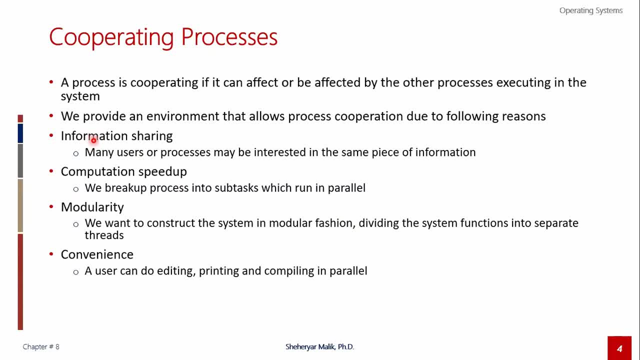 they want to have an access to the same data or same same information. so we share that data or information among multiple problems. we do have physical multi-core or multi-process architecture and we want to have a computation speed up. so what we do, we divide the process into multiple. 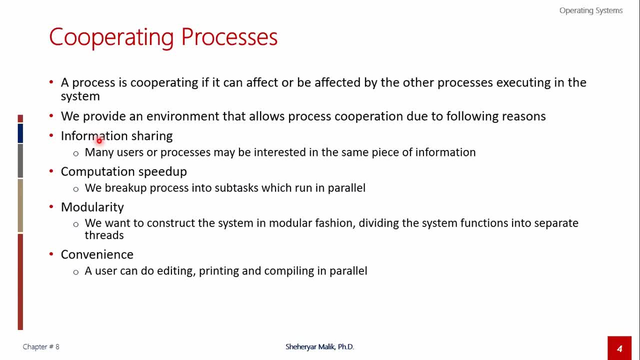 sub tasks and we try to run them. and you know that if you divide it into sub-tasks, even if you don't get physical parallelism, then you still get a lot of benefits. like we talked about last time, that when you divide it into sub-threads and the threads 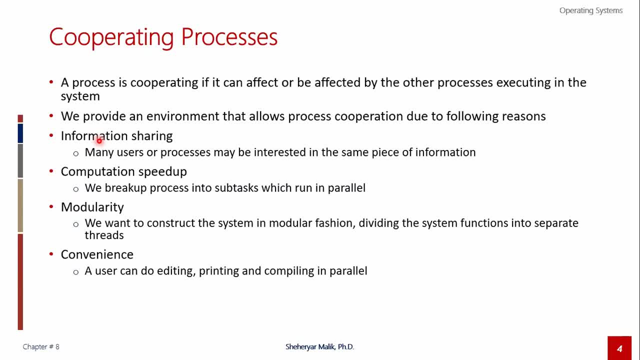 when it comes to blocking, then in the case of blocking the thread belonging to the same process, you can switch it to even one module, and that's where you get the most out of the whole process, and you can see that this is the common thread that you have in the previous process. 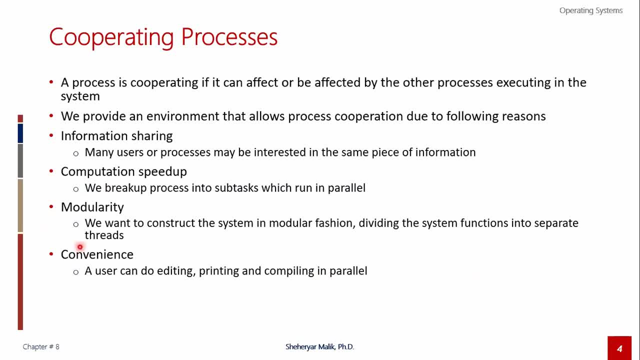 so you are dividing the whole process into multiple threads. this is the reason why your contact switch overhead thing is getting out of control. then when you divide the threads or sub-task- so actually you build the system into a modular way- you let it create more levels of. 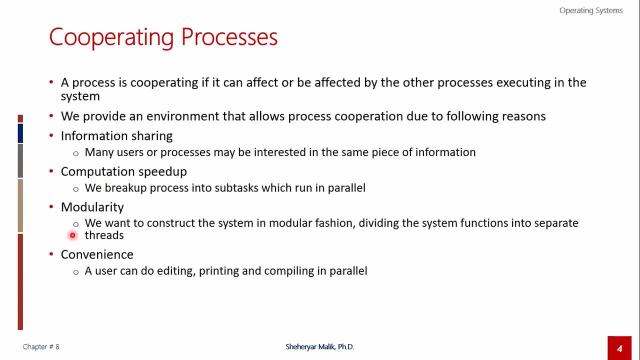 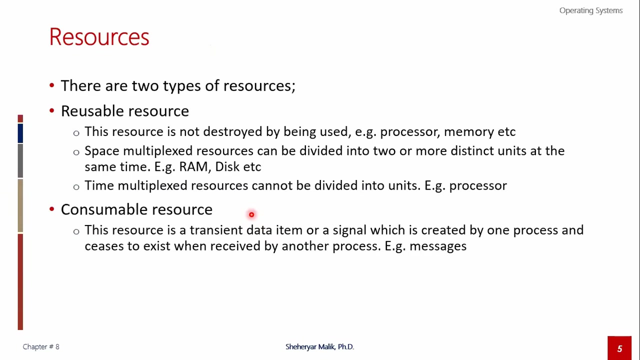 modularization, which makes the code easy to manage, easy to modify, and so you can choose how to modify. it has multiple types of tasks. you can perform the same tasks and when you perform those tasks you can do the editing, spell checking and other stuff in uh. incidentally, related important concept is resources, resources, uh. 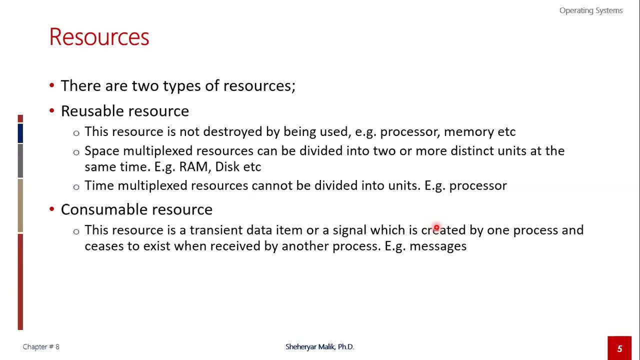 contain so they do not get consumed. just say typically: uh, for example, signals input one to the other other process in form of a screen, so will be uh, consumable resources, ego, space multiplexed, or do so you can: time multiply, space multiplexed, multi-flexed. 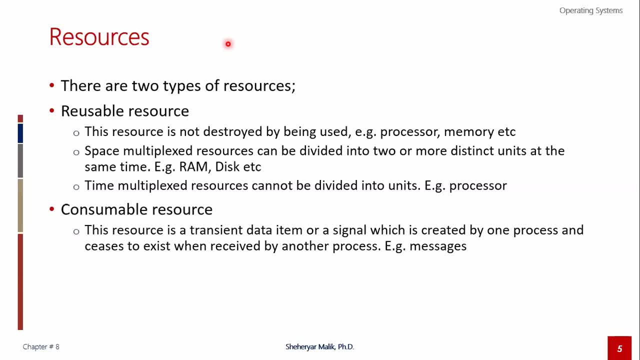 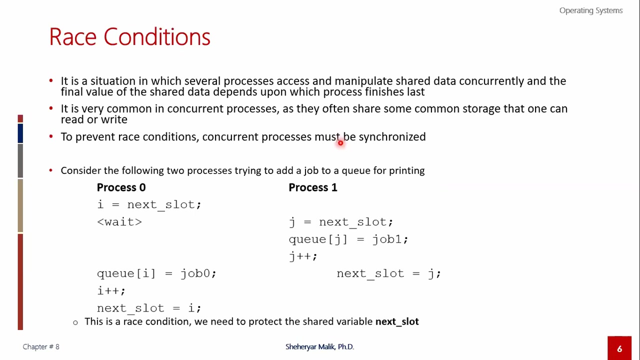 resources at the same time. generally there are multiple processes which are accessing space multiplexes at the same time time. multiplex may get out that you must. uh, mostly just so they are called time multiplex is operating processes nice, or why they are operating? because they are accessing some sort of resources. 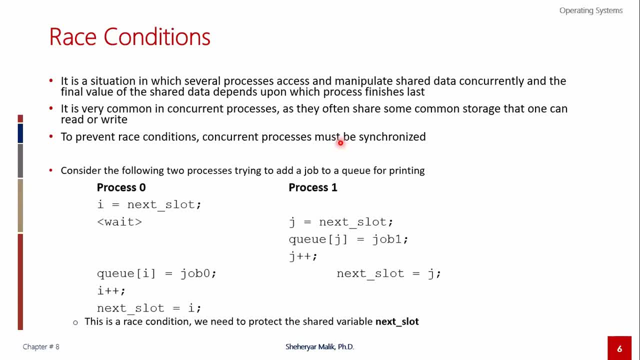 so we do have a race condition. race condition it's a situation in which you do have multiple processes and they are trying to manipulate some sort of a shade data concurrently. so you will end up with your situation, with the situation in which it out, and it is very, very much common in concurrent and cooperating processes. 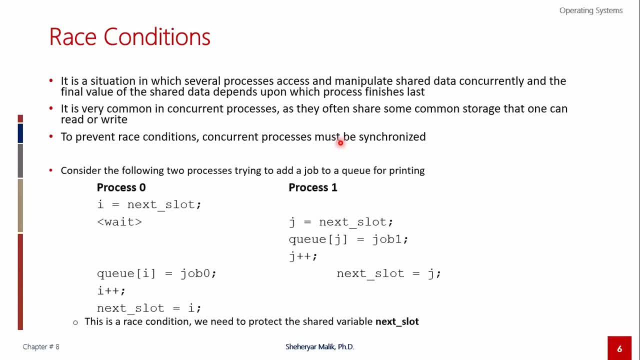 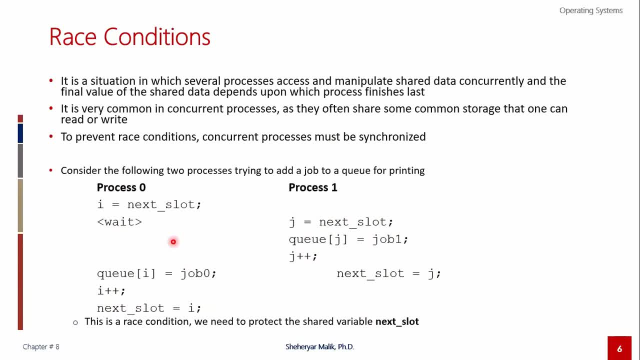 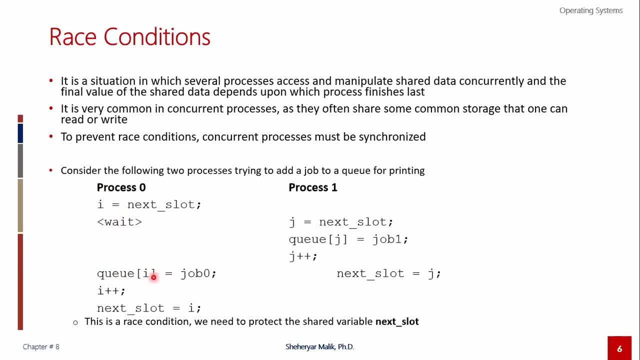 and then Q of i is 5, in 5, which job you have to put or place? job is 0, so you have to put it in Q of 5 and I++ and next slot will be I means next slot is 6. 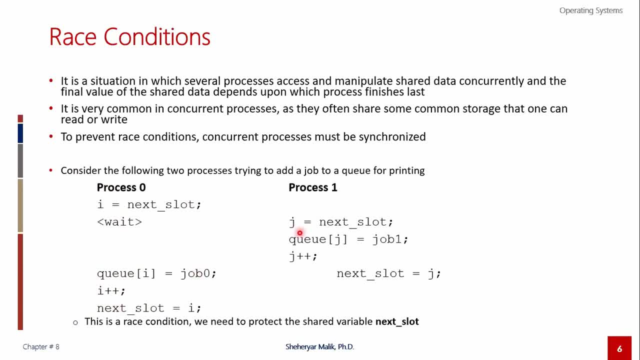 after this, J will process it. Q again: QJ will be your share. when J will process it, J will see what is the value of next slot. what should J get? J should get 6 and Q of. J will put 1 in 6. 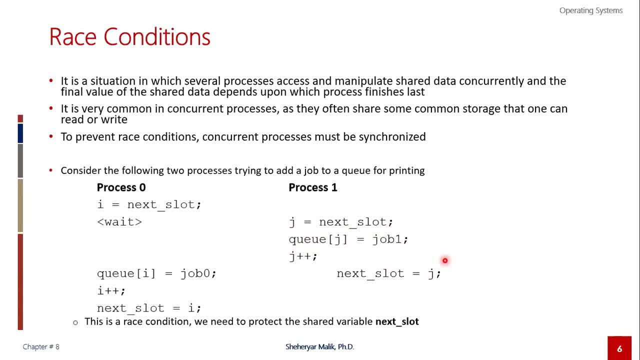 and J++ will send J in next slot. but if it is not synchronized, as you can see the situation here, because J is waiting and at this time J has accessed it, if you understand it as timeline from here in vertical, so you can see that I took next slot. 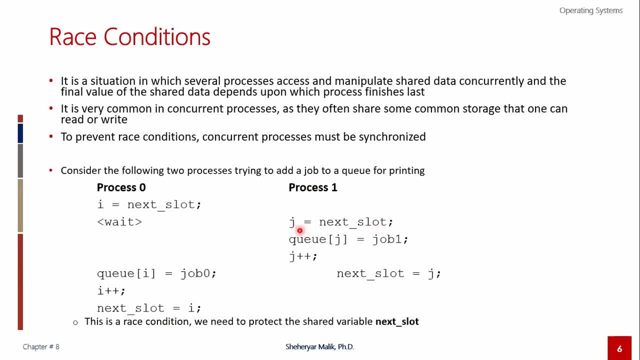 what value did I get 5? what did J get 5? ok, here, when it did this, in which will it put in 5? but before this, J got the value of next slot and it got 5. and when it put job 1 in it, where will it place job 1?? 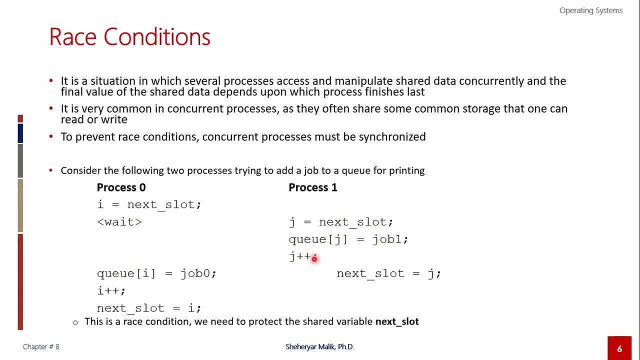 in 5, and after that J is doing plus, plus and then J is doing next slot, so it will make next slot 6, while what will it get here? Q of i is this, and it will get job 0, so it will get Q of i here also. 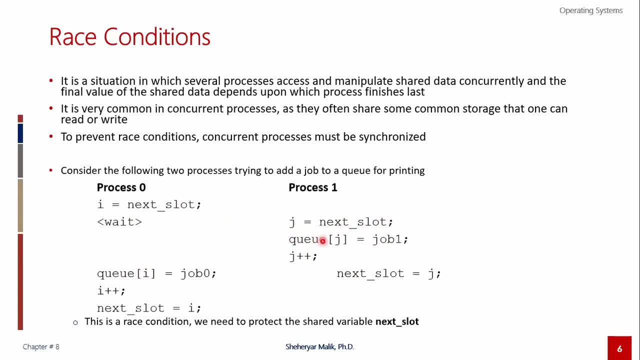 it will get 5. so 5 already had job 1. it should go to next instead of next. it placed job 0 in same place and if J did i++, what would be i's value? it would be 5. it will do 6. 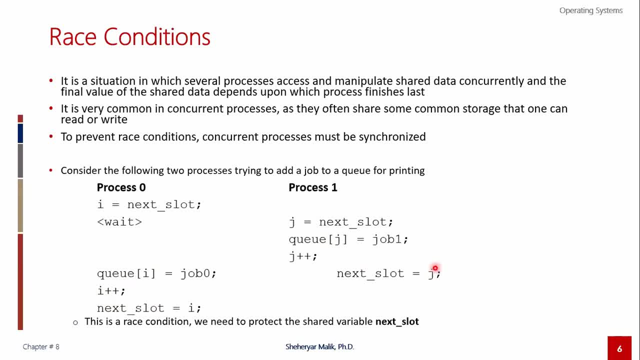 and what will next slot do? it will do 6. it has already done 6. then it did 6E again, due to which all the work is done, because one is overriding and the other value of the next slot is also wrong. two people have processed. before starting, it was 5. 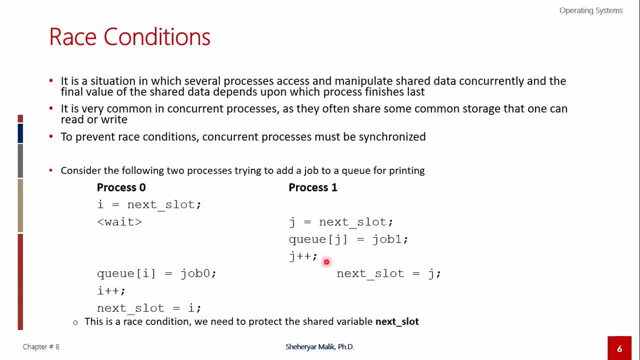 when two people have processed, then both should have one separate space and the value of the next slot should be incremented by 2- first one does it, then the other does it, and it should be 7, whereas in this situation the value of the next slot is 6. 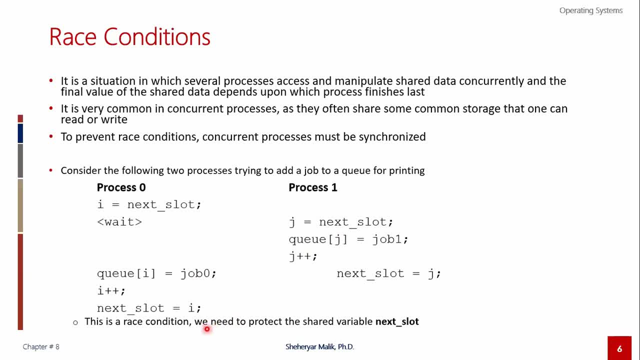 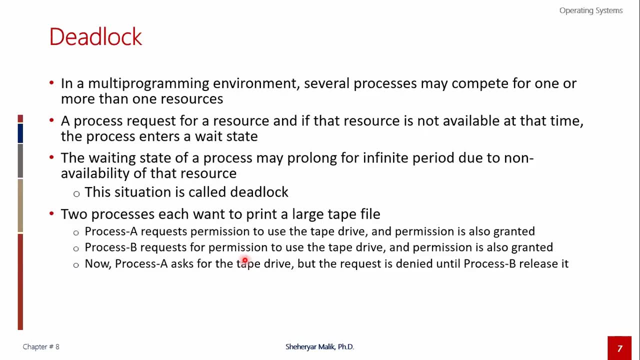 so whatever will come next, it should be placed in 6. so if these two are repeated again, then again same situation. this is a problem. what is the problem here? the main problem is when it came here and went for the reading, because it is doing some sort of processing. 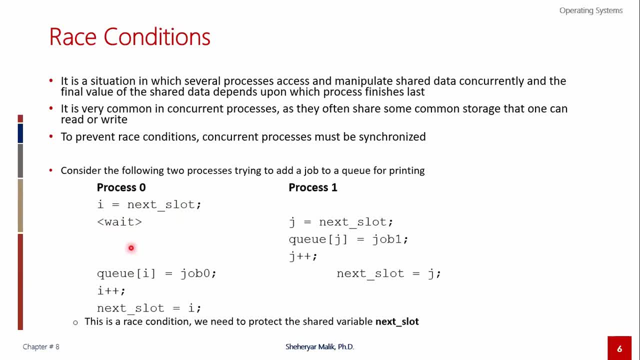 onto this shared thing, what is shared. next slot, next slot is really playing an important role. so next slot needs to be synchronized. who has to access it? its mechanism: if we use this mechanism for it, you have to locate it, you have to use a locking mechanism. 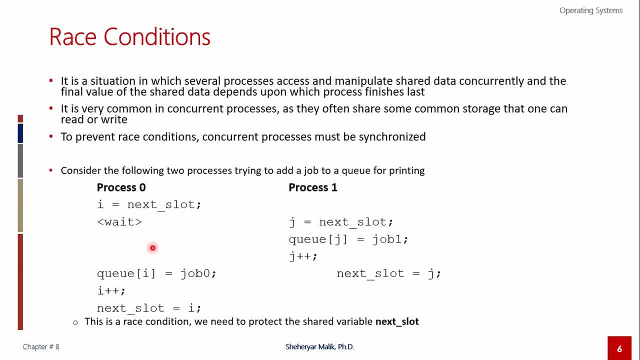 until and unless your your your sorry- next slot, you have to use a locking mechanism for it. so what will this locking mechanism do? it will lock this next slot so that j can't access this next slot, because if it has accessed it then it has a suits. 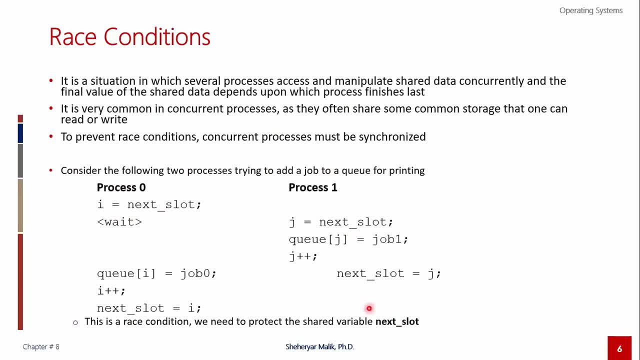 see what is the problem here. there are two processes. now we will talk about shared variable. now we will talk about cooperating process. this is a separate process. this is a separate process. let's say, a queue is made, like jobs are placed in unix based system. you have to perform a job. 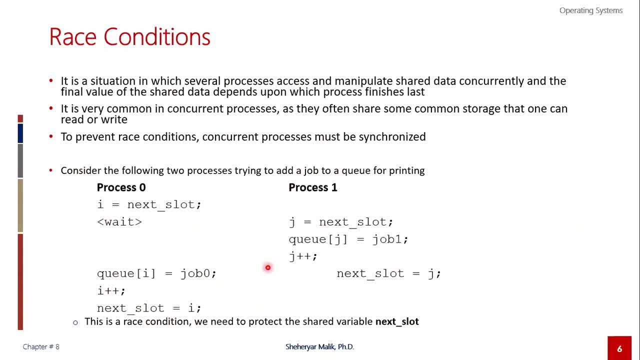 this is shared queue. in that shared queue you have to place a job. let's say you manufacture something and you place in a running queue. so two things in queue can't come in same place separately, separately, in which this is going to be told to us by next lot. 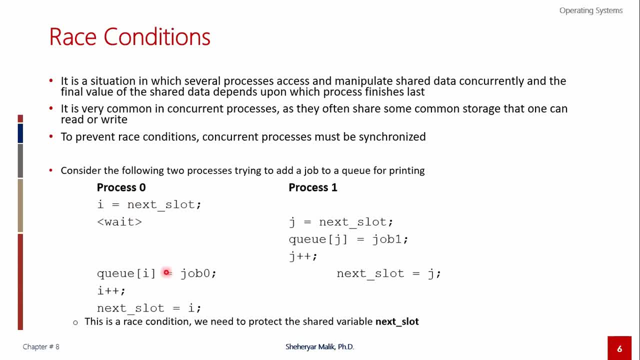 next lot tells us in which to place i is index value, this process and its local variable j. it takes its value. it says next lot. it takes its value. so it tells us its value is 5. before this we will assume that it was 5, 5 slots. 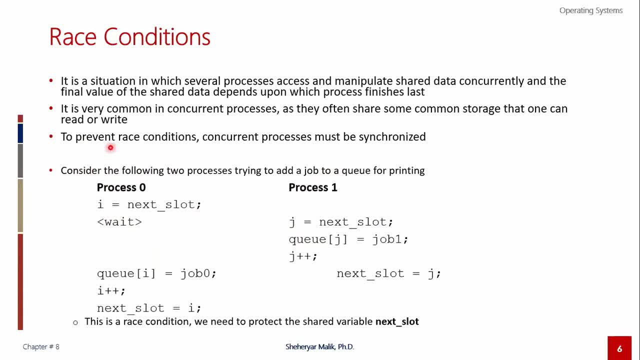 0 to 4 were filled. so 5th slot was empty. so it says 5 is coming, so it gets its value. so next slot is shared value. what is available after this? he has to wait. he had some waiting time to do the process in j case. 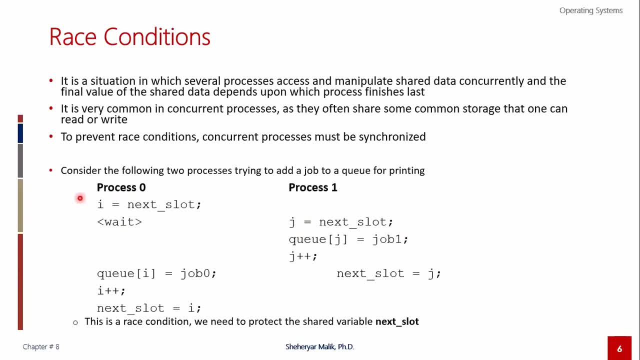 in j case, j also accessed next lot value. now, time is running vertically, so this is your time. this is your time, to assume that this is your time. ok, these two concurrent processes are executing together on two processors, so j also took next lot's value. what did i get? 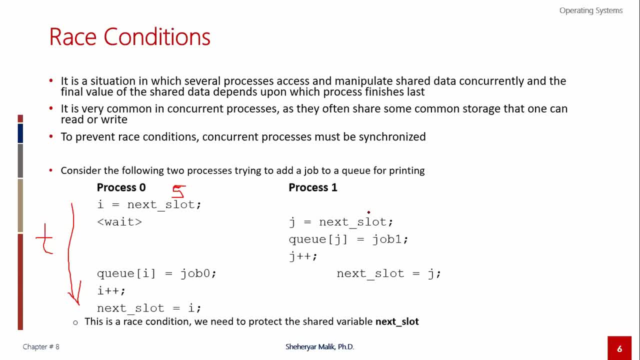 what was here 5. So what will he get? 5. Means what will be the value of j 5. This will go in the weight Here. when he had to produce a job, he placed it in this q. 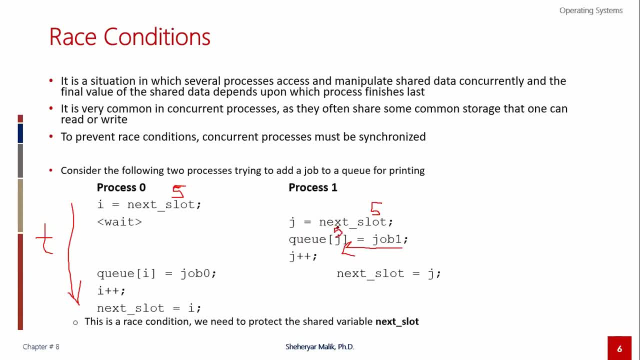 So where will he place it in q? What is the value of j 5.? After this, what did he do by doing j++ 6. Here, when he processed it in q, he had taken the value of i. 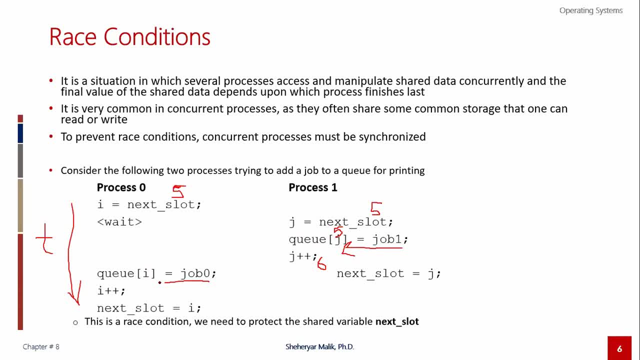 So when he has to place this job, where will he place it? What is the value of i? The value of i is also 5.. So where will he place it? He placed it earlier. Where did he place job 1?? In which element of q? In shared q? In fifth? 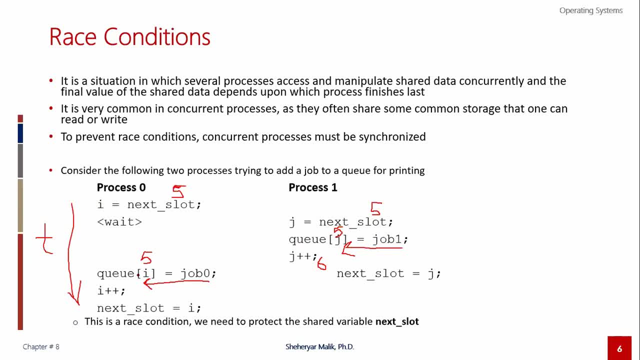 Where did he place it? He also placed it in fifth. Whereas what will be the value of j? It should be in next, So he placed it in fifth And when he did i++ he also placed it in sixth. Here before this, he processed it and the value of j was 6.. 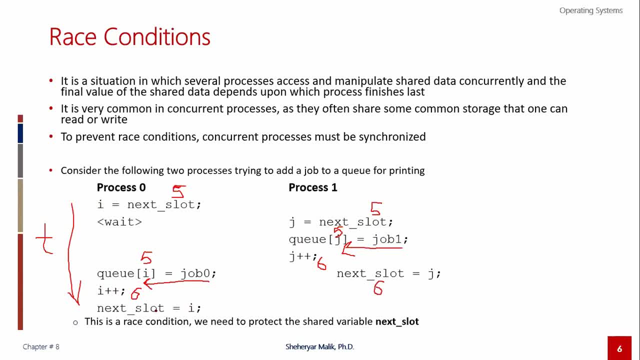 What will he do with the next dot? He placed it in sixth. What will he do with the value of j? He also placed it in sixth. What will he do with the next dot? He placed it in sixth. Whereas, what will be the value of the next dot after the execution of these two? 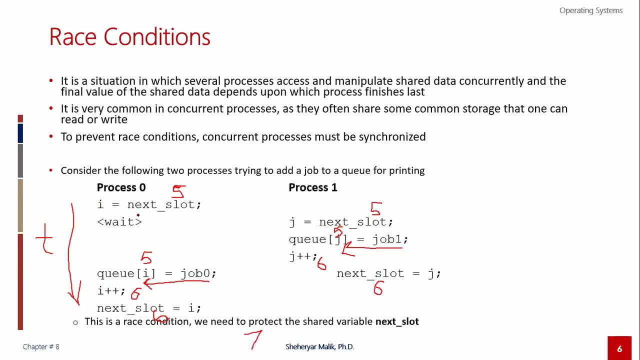 7.. So why is there a problem? Because any one of the two faces is accessing the shared thing, So you cannot do this. What is the method of this? Whenever you will access the shared, you will do locking for it. 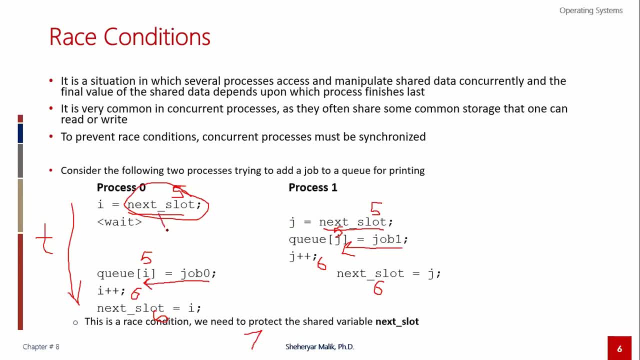 What is locking? When i has accessed the next dot and now it has to perform the operation on the base of this shared queue, then you have to lock this variable Now. no one else will access it. Okay, You have accessed it. 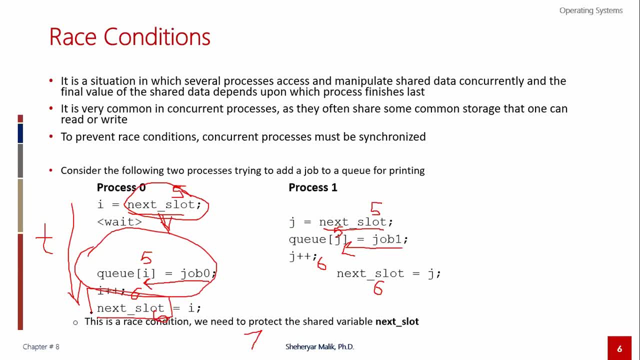 You have updated its value. After this, you release its lock. When you release it, what value will it get now? When it will get after release? it cannot be executed at the same time. It has to wait. It is a cooperating process. It has to wait. 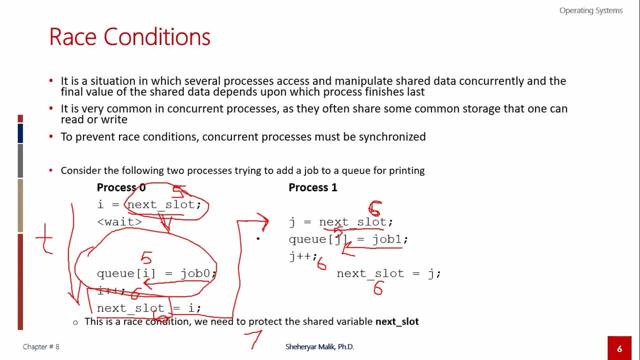 What value will it get? It will get 6.. And then where will the job 1 go? It will go to 6.. J plus 2 will be 7.. What will be the value of J 7.. Now, this is fine. 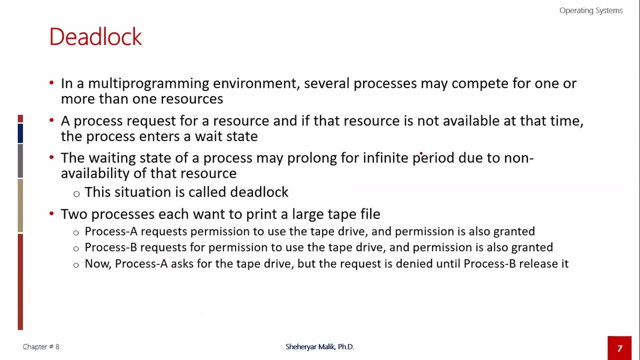 But if you will not do any synchronization on it, if you will not do locking, if there will not be any mechanism, then this is a problem. It is fine. Now, what is the problem? because of this, You can access a shared thing. 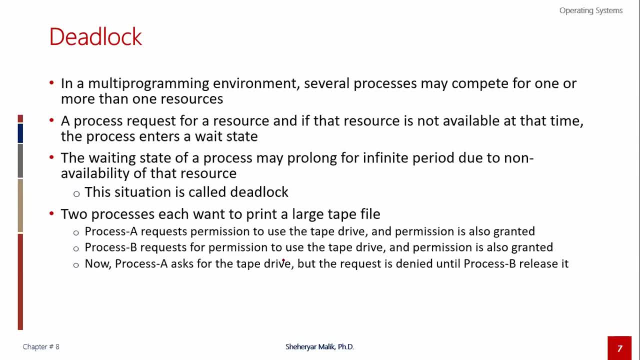 without locking, without synchronization. if you will try to access multiple together, then you can have a deadlock condition. What is a deadlock? You are going to a chowk. It is a very common example: If you do not have your signals. 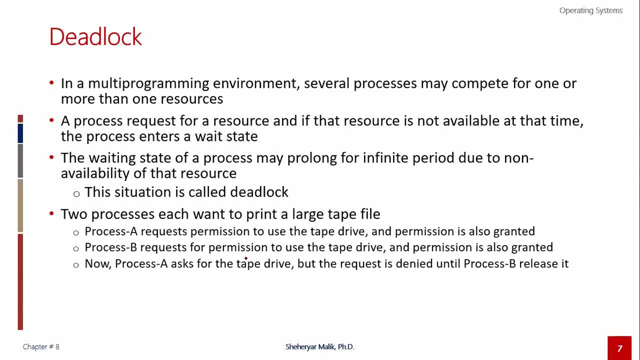 then what will happen? If you are in any country in the world, you will be in a deadlock, Your traffic will be jammed. If there is no police and the signal is off, then what happens? You can see that Everyone tries to cross that shared chowk. 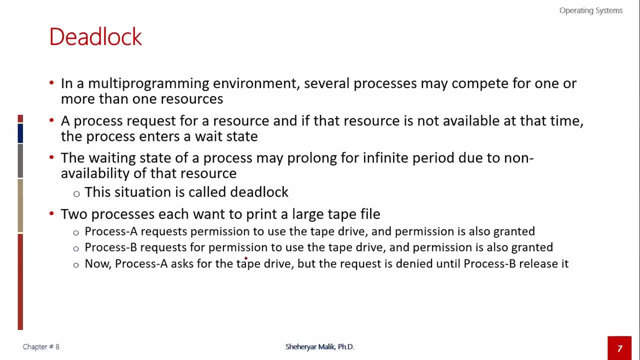 That chowk is shared, Everyone tries to access that chowk at the same time. If there are no signals, then what does the signal do? It avoids the deadlock. It gives access to one side at a time. For others, it is locked. 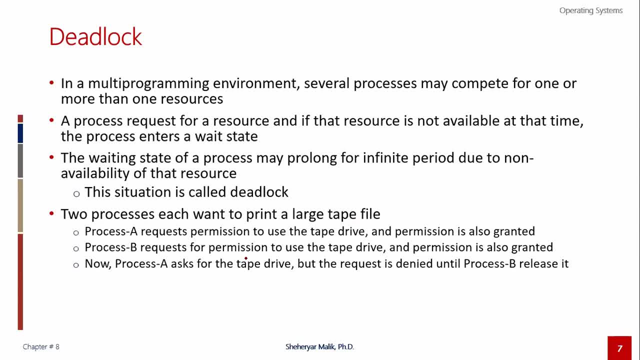 Red signal is a locking mechanism. It locks, It passes through one side at a time And for others it stops the shared resource. Similarly, if you try to use all the artists, all the RAMs, all the CPUs, then you are going to have a power. 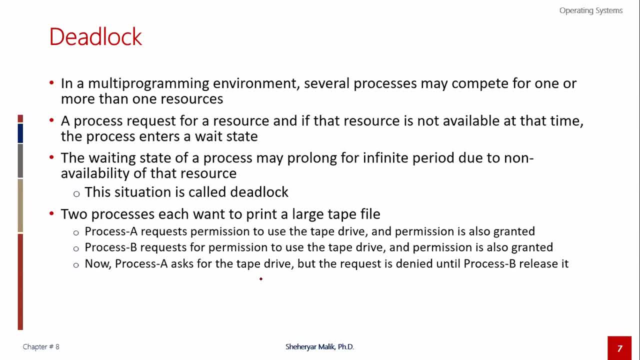 You cannot do that, So it becomes a deadlock. The second situation of a deadlock is that we did locking. We said that the way to avoid a deadlock is to do locking, But the locking was such that the one who was given the resource did not leave. 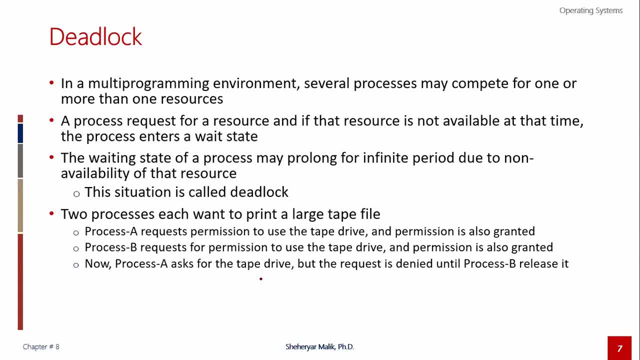 The one who was given the resource was permanently locked. The same happens at the chowk. Sometimes the sergeant opens the traffic of one side for a very long time. Now others have to wait a lot, Let's say, if he opens only one side. 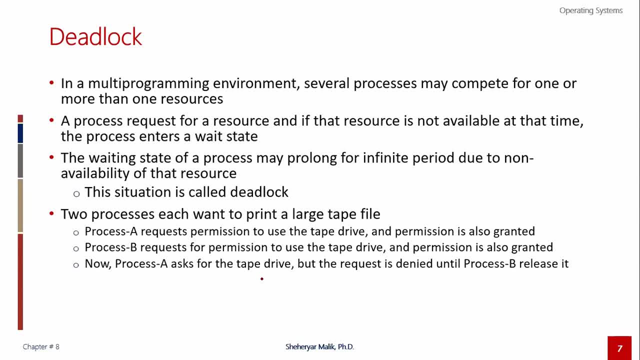 then what will happen for others? The chowk will be open. There is not a practical deadlock, But this is a deadlock for the others. So this situation is called starvation. This is the situation of a deadlock In which some people get the resource. 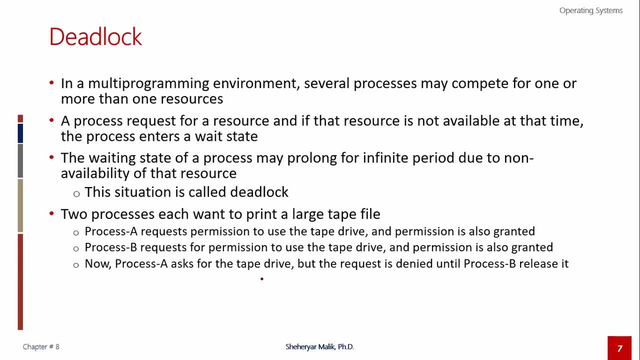 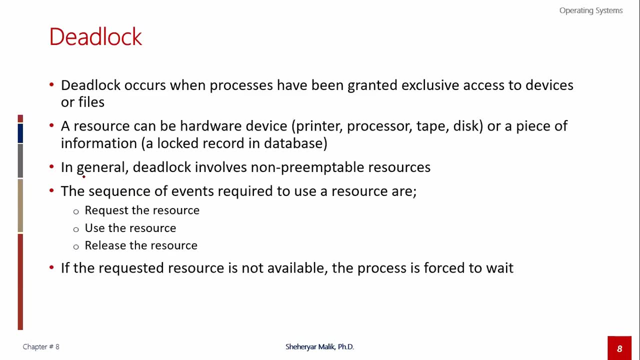 but others do not get it. That is called starvation. So this is how it is. You have a circular deadlock. One person gets the resource and the other wants it, So it becomes a deadlock. So these are called deadlocks. 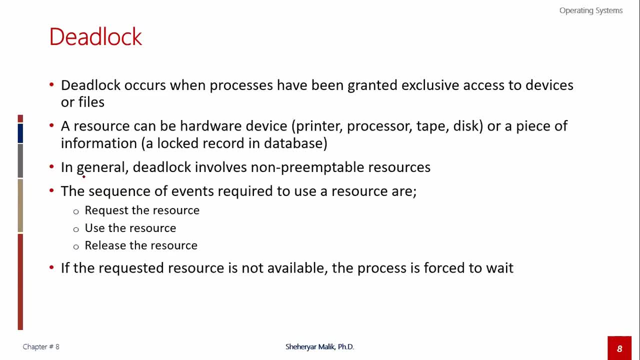 So why? generally the deadlock occurs? Because you give an exclusive access to the devices, files, shared resources. So when you give exclusive access, it becomes a deadlock. This can be for hardware or for software. Multiple applications are trying to share. 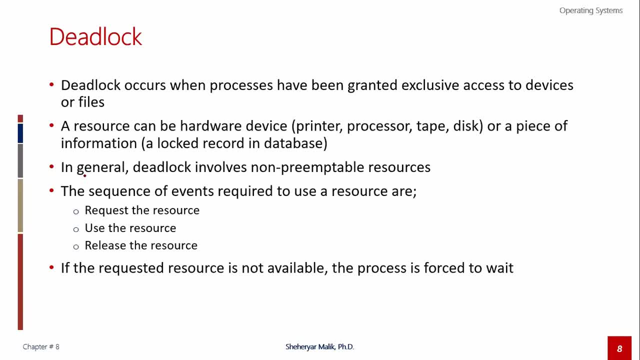 the same data. You are accessing your bank records, You have issued a cheque, You are standing on an ATM and you are doing an online transaction. So if you try to access records from three places, you can have a deadlock, And how big an issue can be in this. 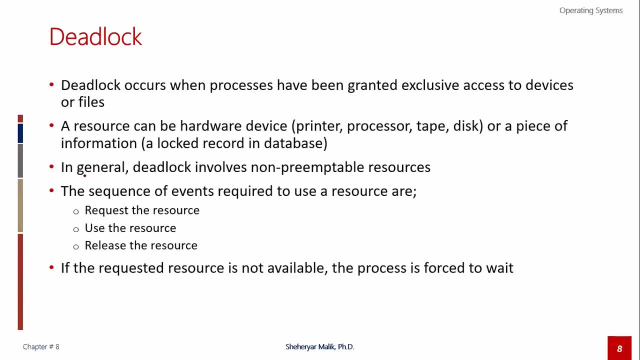 If the record is not locked and you have issued a cheque for 15,000. You are withdrawing from an ATM for 10,000. And you want to transfer for 20,000 or 18,000 online, If all three are at the same time. 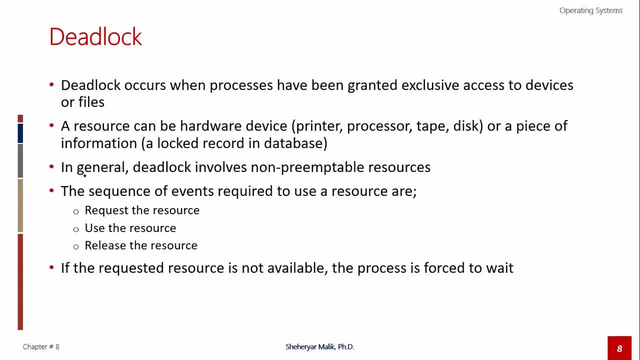 what will be the first task of all three? What will be the first checking? What is the account balance? So the account balance is 20,000.. All three have checked simultaneously. After checking 20,000,, a simple transaction takes place. 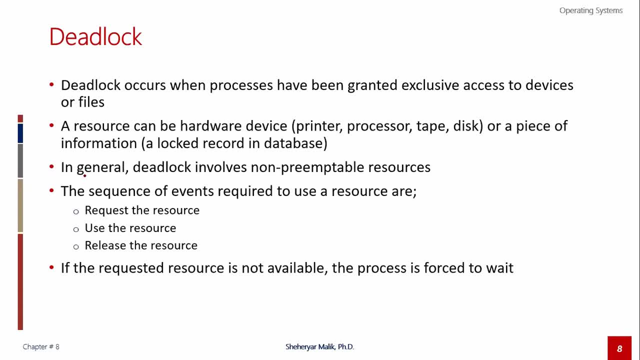 For all three transactions it was less than 20,000.. But in a nutshell, how much was it? 10,001, 15,001 and 18,001.. So the total is 43,000 rupees. 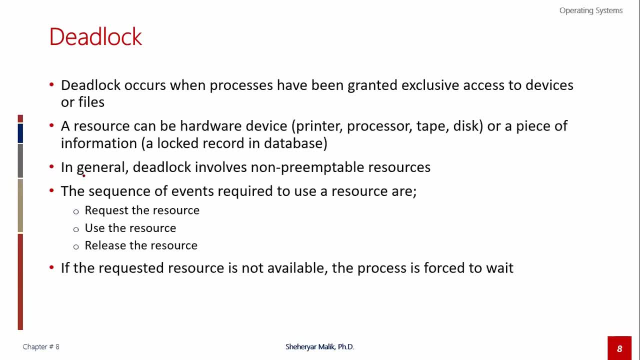 While the total was 20,000.. So it should be locked Because it is a database, So it is a database's record locking So one of your records is accessed at a time, Otherwise it creates a problem. 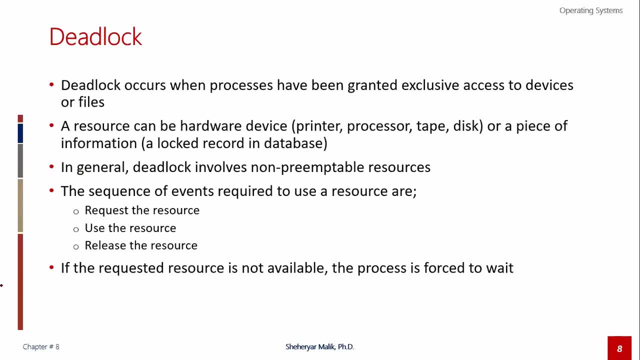 And why do deadlocks happen? often, Especially the case of starvation, is a case of non-preemptible resources. Deadlock happens with you. Let's say you have to take a print And one person has sent 300 prints, So a deadlock or starvation situation. 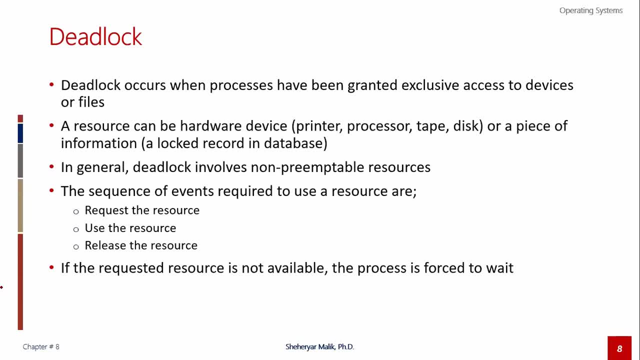 is created that you cannot access it. It takes a lot of time. So generally the sequence to access any resource is that you first request the resource- I need to have this resource- Then you use that resource And then you release that resource. 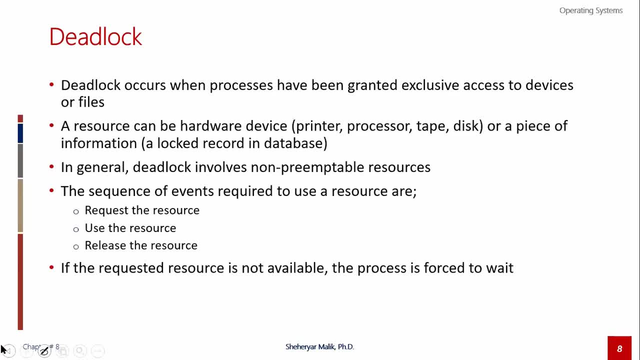 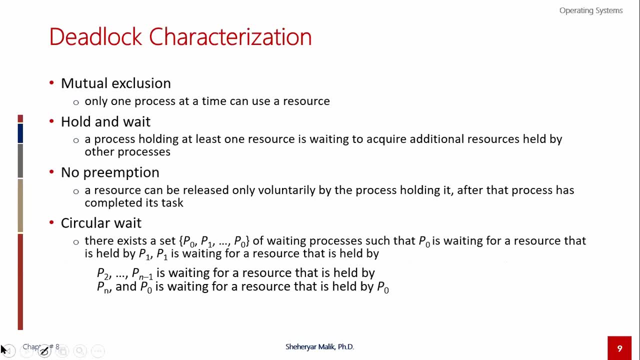 According to this, we have a mechanism to handle the deadlock. If we look at the deadlock characterization, there is a great mechanism to avoid the deadlock That is called mutual exclusion. But that mutual exclusion can result in a starvation as well, Because 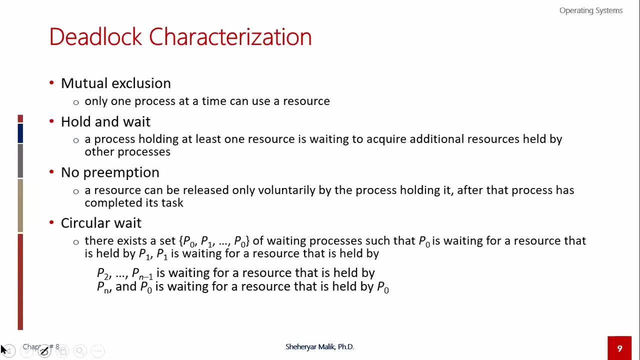 what we say. due to mutual exclusion, probability and statistics are different. You must have studied mutually exclusive events. What are those? Can you tell us what are mutually exclusive events? More than one participants? No, more than one participants. But what is a mutually exclusive event? 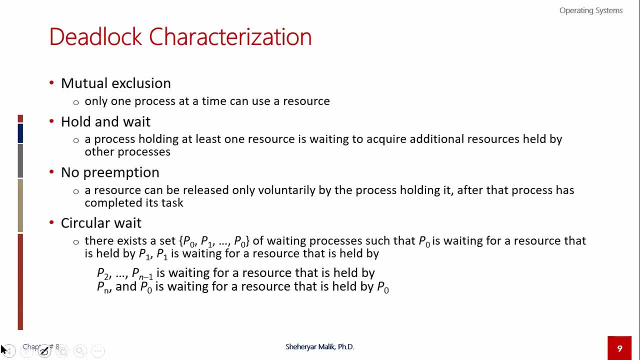 Organized by more than one participants. No, no, Mutually exclusive is: if you have multiple options, only one can enter at one time. Like you roll a dice In one moment. there can be only one phase: 1,, 2,, 3,, 4,, 5 or 6.. 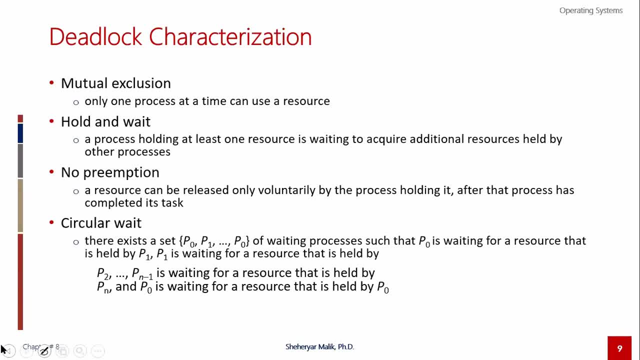 That is called mutually exclusive. And similarly, if you apply mutual exclusion in one moment in one process, you can use a mutual exclusion So that becomes a mutual exclusion. So this is a mechanism to which we handle, But this can create a deadlock. 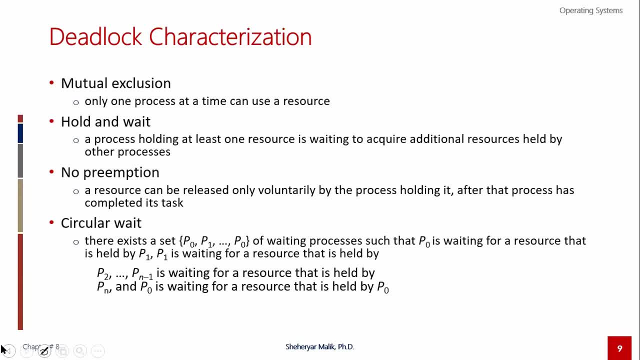 until it is indefinite. If you give mutual exclusion to one resource and not to others, then that creates a deadlock. Then hold and wait. What is hold and wait? A process needs a resource. This is P1. And this is resource 1.. 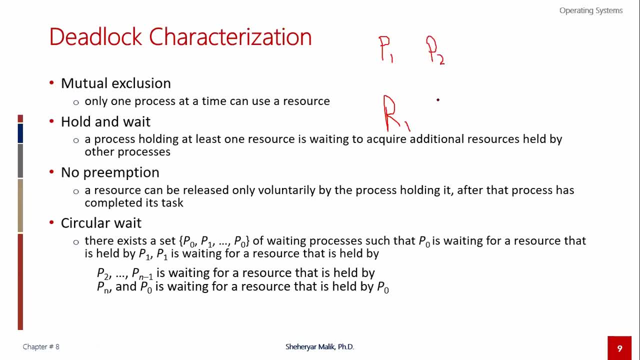 And this is P2.. And this is resource 2.. This is another resource, So P1 has also held this resource And he wants this resource to also be different, So he is also using P2.. One resource is hold and 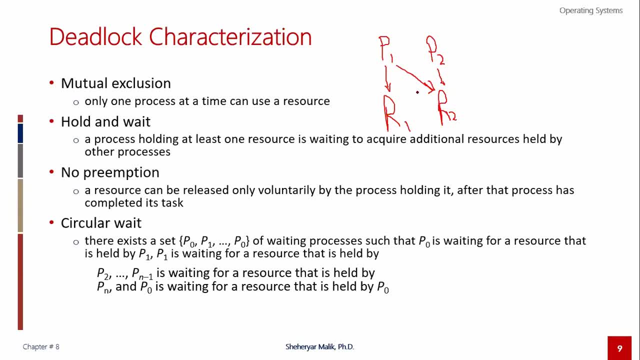 the other is wait, So that is called hold and wait. If this gets disconnected, please join again. Thank you After this, no preemption What I just told you: When a process does not complete its work, it leaves the resource. 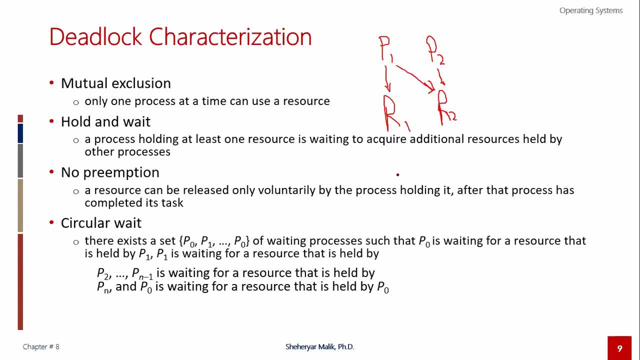 So that is a resource preemption, No preemption. You are not preempting. You have given the same resource non-preemptable resources. Please keep on accessing this. Then is circular wait. This is the most interesting In this. the same situation is P3.. 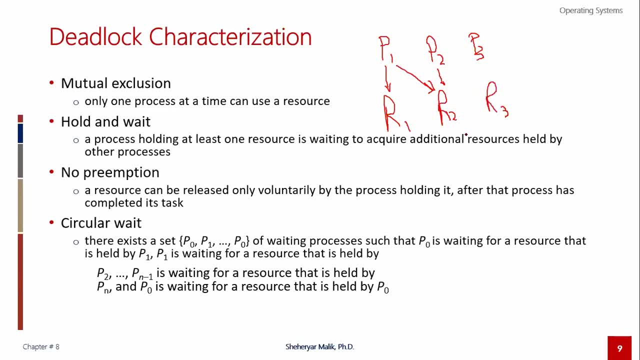 And this is another resource: R3, R1.. P2 has held this, And who is doing the wait? R3.. And P3 has held this, And who is doing the wait? R1.. So this is what. 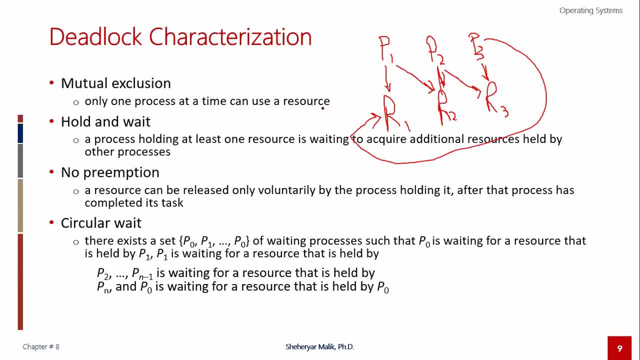 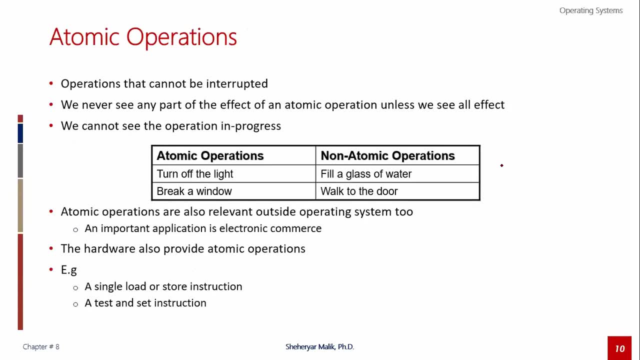 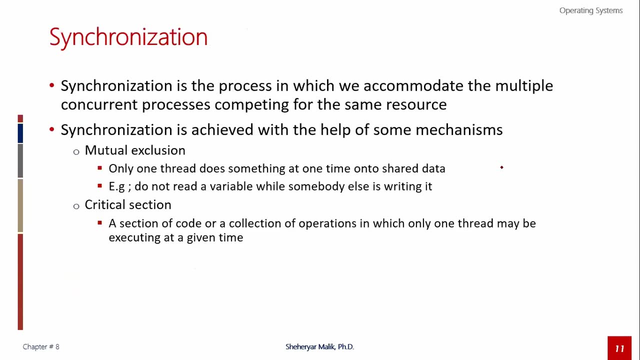 Circular wait. Now this is completely deadlocked. No one is able to access any resource And he is waiting for the other resource. Ok, So what we do for this? We try to synchronization. We try to synchronization with the help of: 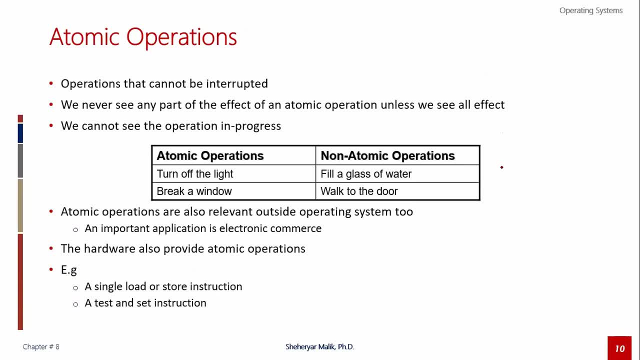 some atomic operation. What is atomic operation? Atom? what is atom? As far as a long, very old definition is concerned, Atom is the smallest particle of the universe, Which is an incorrect definition. now, Atom is the smallest particle of the universe. 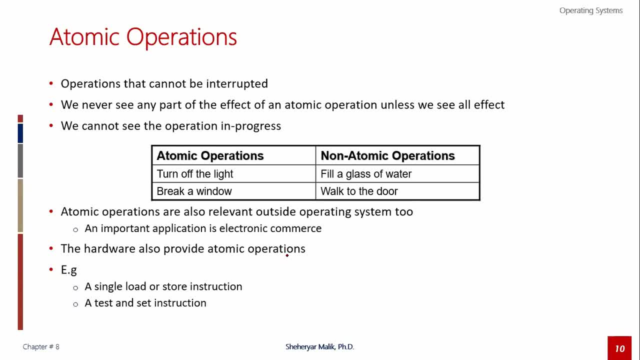 And we found more particles as well, The smallest. they were used for explosions and operations. So anyways, Atom or atomic has become a property. Ok, In literature Atomic is what Which is indivisible, So operation that cannot be interrupted. 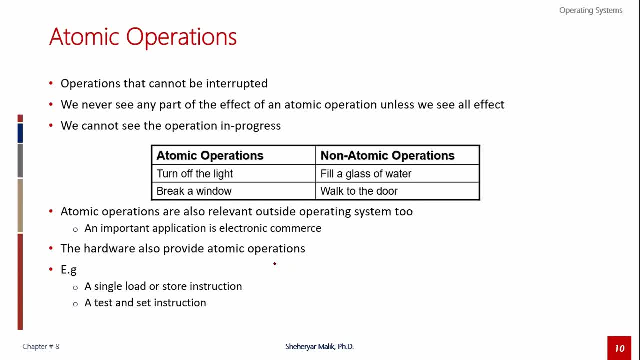 is called atomic operation. For example, in general in light you turn off the light, So now this is atomic operation, You cannot stop it. Similarly, you hit something on the window And the window is closed, But in non-atomic. 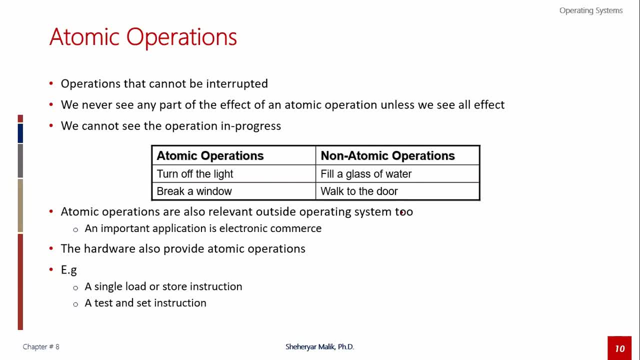 you are filling a glass of water. You can stop halfway. You can stop at 70%, Walk to the door. You are walking towards the door, You can stop in between. So in hardware you have atomic operation. It is a multiple combination. 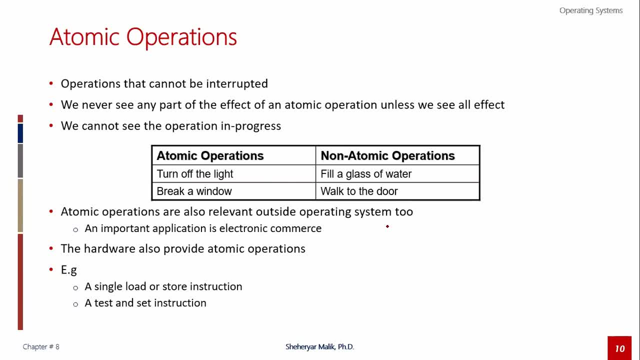 of two instructions, For example load and store instruction. You might have used this instruction One single load and store instruction. That is atomic. You cannot interrupt in between. This is test and set instruction. You test the variable, Now comes the synchronization. 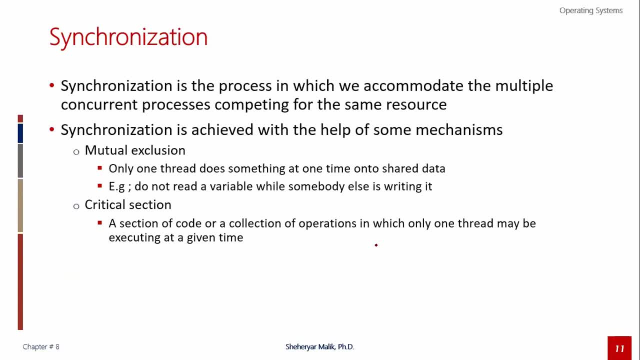 What is synchronization? So this cooperating process is okay. We are having deadlocks, We have a race condition Due to race condition, you can have deadlocks, You can have starvation. So what we have to do is we have to provide a synchronization mechanism. 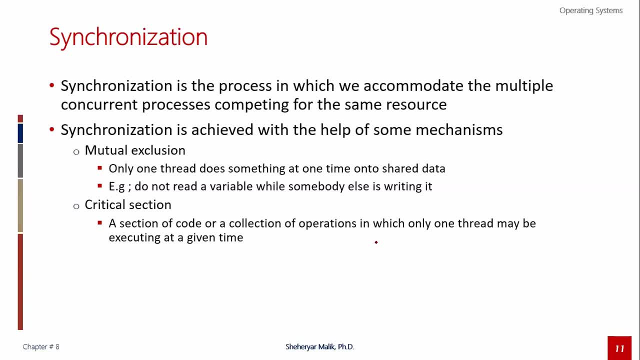 What synchronization does? it provides a mechanism which de-facilitates the concurrent or competing clock Which is for the same resource To compete. So to achieve synchronization, we do either the mutual exclusion or we provide a critical section. These are the two concepts. 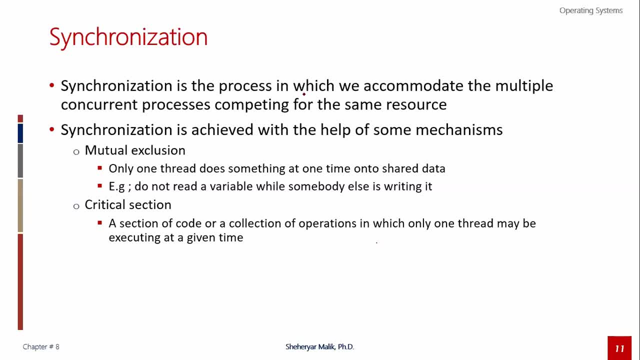 What is mutual exclusion? We talked about this earlier. At one time, only one task or a sub-task or a process performs something onto the shared data. What does it mean When someone is accessing the shared data we are not going to access that? 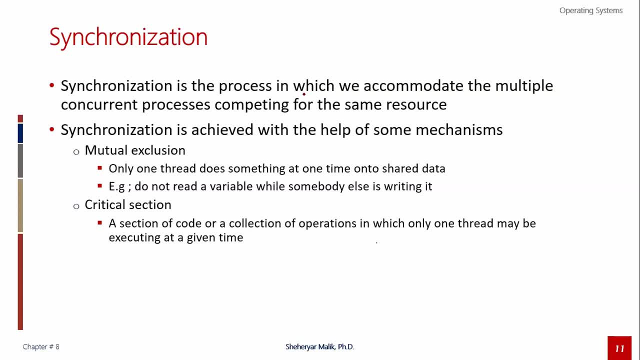 We are not going to access that. We are not going to access that. And what is critical section? That piece of code that you have written in that code, that portion, that area which is sensitive, or where you access that shared thing. 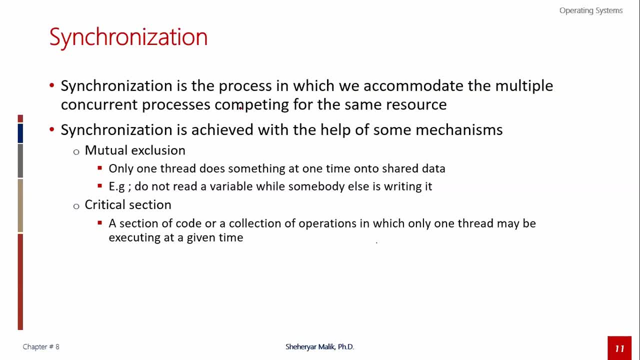 That is called critical section or critical region, Understand. So you do not access the shared thing, You have accessed that shared thing somewhere, So that is called a critical section. So that is called a critical section. And what is mutual exclusion? 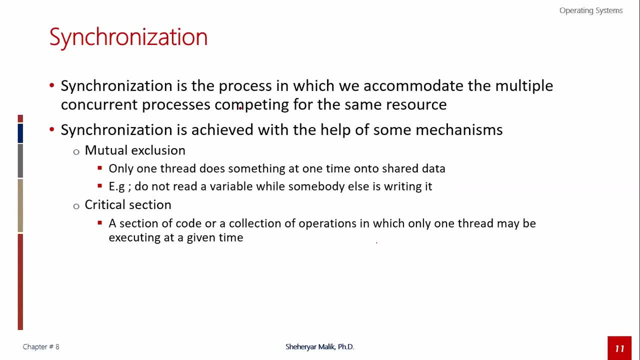 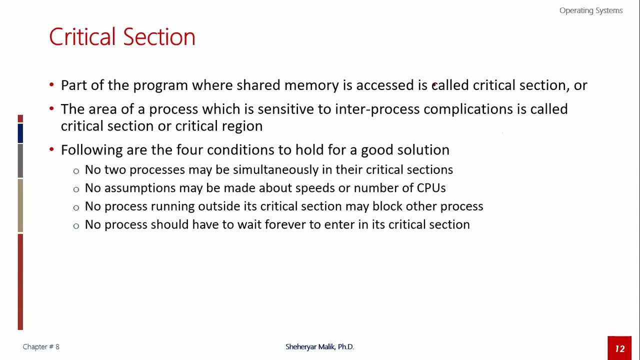 At one time, someone is accessing the shared data, So we use the mixture of these two. So what is critical section? Where you are accessing the shared memory, That is called critical section. Shared data can be memory or anything else. 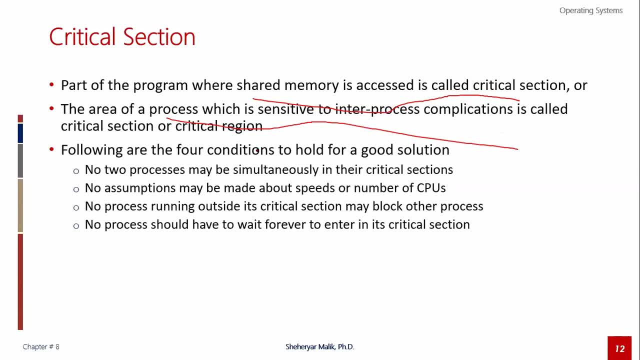 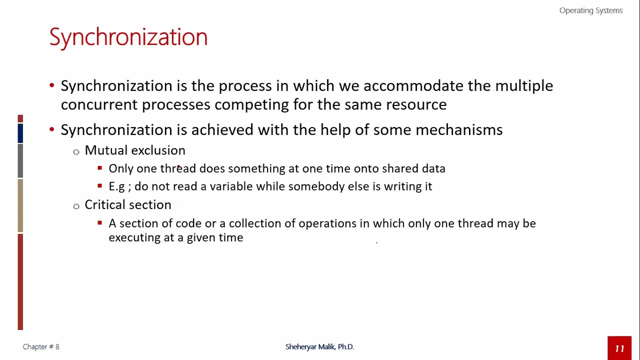 And the area of process which is sensitive to inter-process complication. We implement this with mutual exclusion. We say that at one time, one process will take its critical section, Not more than one critical section. This is the main thing. Mutual exclusion is applied to critical section. 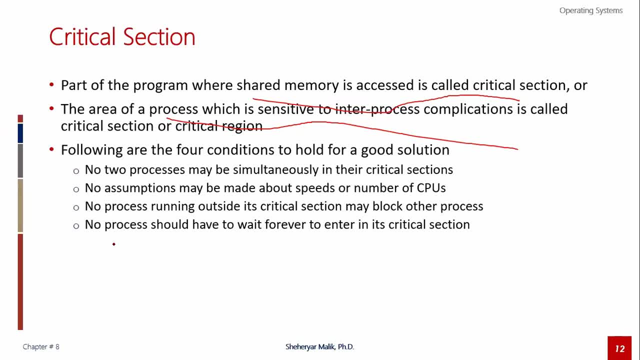 One will be critical section. Second, that critical section is small, It is limited. Only that thing is in critical section which is relevant. You have read advanced computer programming. You have done exception handling. So what do you do For exception? 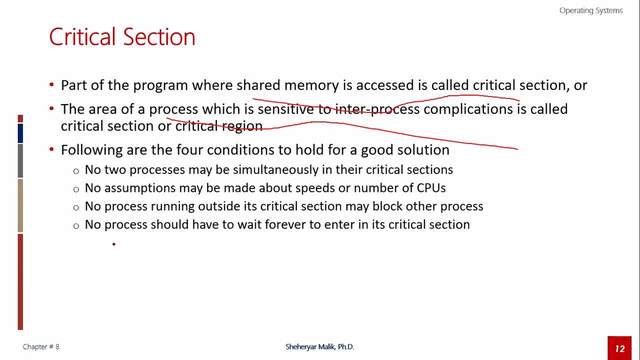 what do you put sensitive things in Try block. But what is the recommendation for that? Only that much code should be put in try block which is subjective for exception. Where there can be exception, there will be an effect of exception. Only that code should be put in try block. 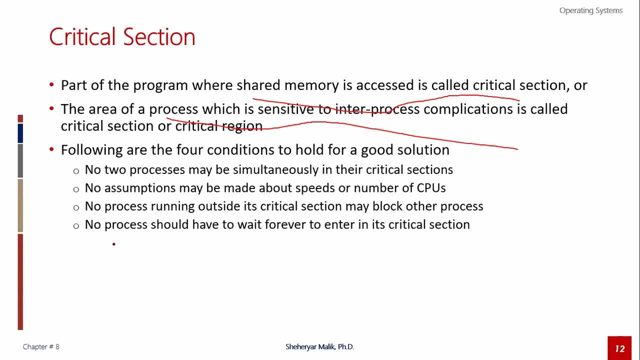 Because if you put more code and there is an exception and there is a code below which is irrelevant, then you will have a problem. The code which will be the exception will not be executed. That is why you should make try block smaller and smaller. 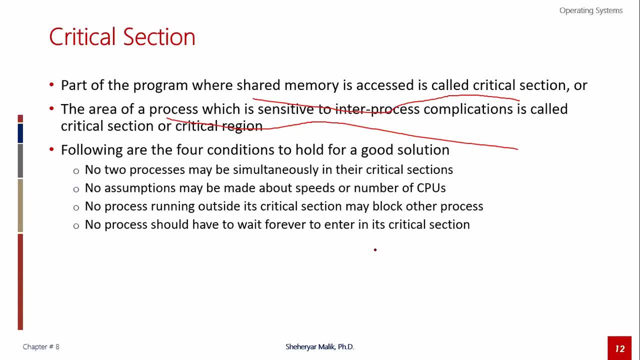 Similar is for critical section. In critical section only that code will come which will give access to shared data. So keep its size minimum. So a good solution is what following four conditions hold: No two processes may be simultaneously in the critical section. 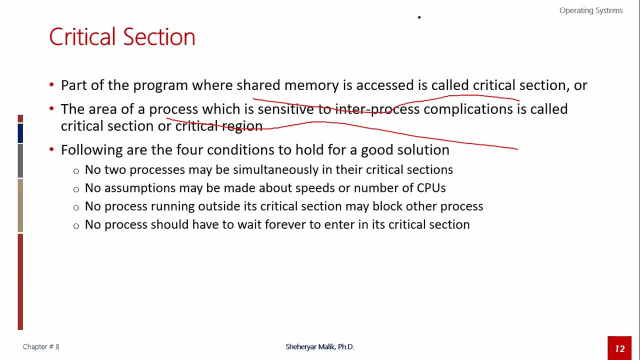 In one time. no two processes will be in critical section. Okay, So what will happen in critical section, The part of the program which is sensitive for your accessing the shared data, Where you have shared data and you want to access the shared data? 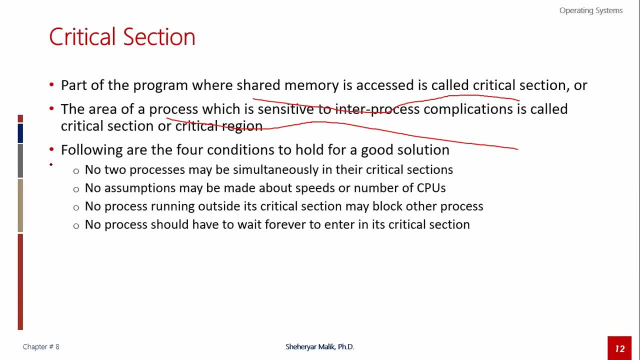 We discussed that it should be as small as possible And the area where we want to access the shared data. So what are the four conditions? Number one: only one process in one critical section. No two processes may be simultaneously in critical section. 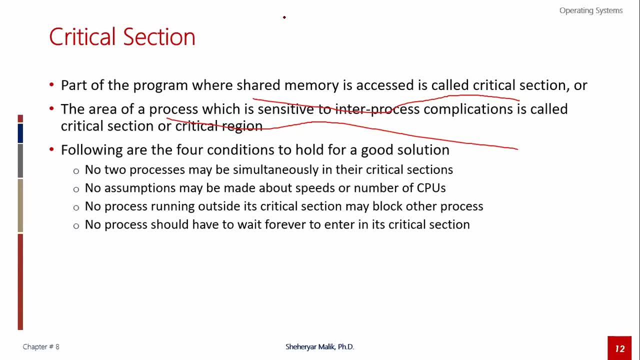 Means. we are employing mutual exclusion here. Number two: no exemption may be made about speed and number of CPUs. How many CPUs are there? What is the speed? No process running outside its critical section may block other processes. Now what will happen? 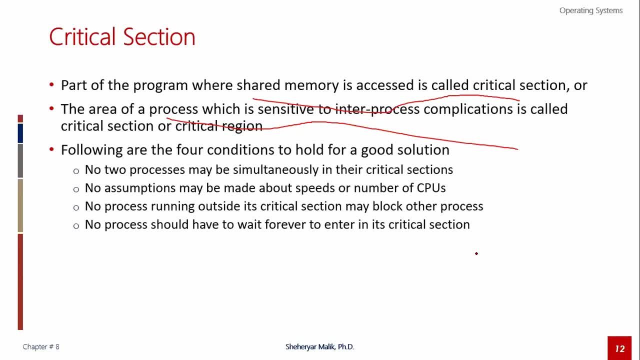 When we will allow one in one time. because of that one, those who want to access the rest will get blocked. But the process which is coming out of that section will not block other processes, And for this both cases are same. 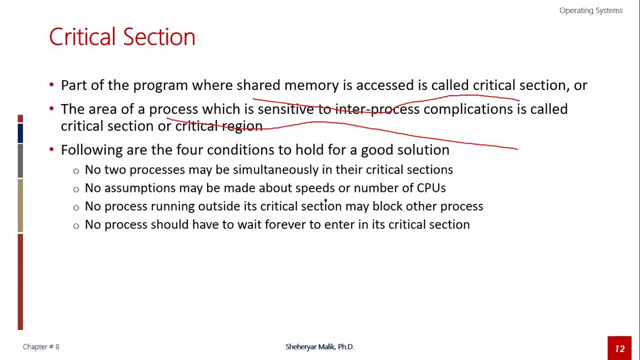 One comes out of critical section and does not block other processes, And the other critical section, which you have made so big by adding irrelevant things, will block other processes. So no process should have to wait forever to enter its critical section because there is no starvation. 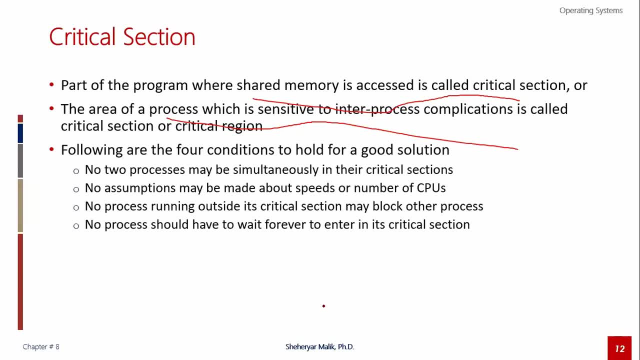 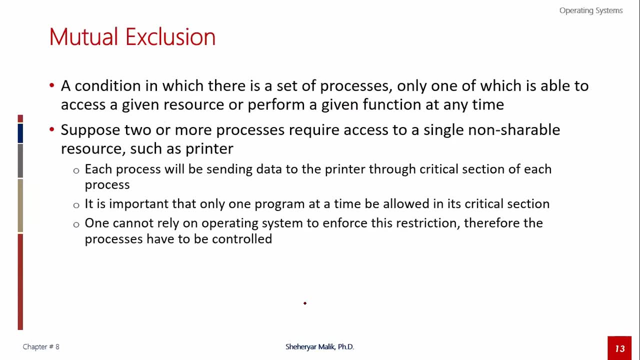 These are the processes which we wait a lot to enter so that nothing will be completely exclusive access, So mutual exclusion. we have discussed What is mutual exclusion, Where we are having multiple set of processes so only one of them is going to get an access to the shared resource. 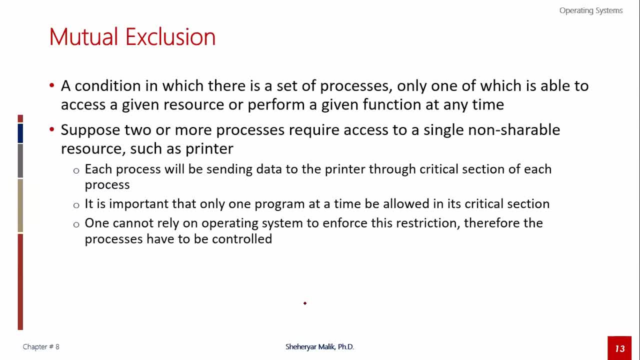 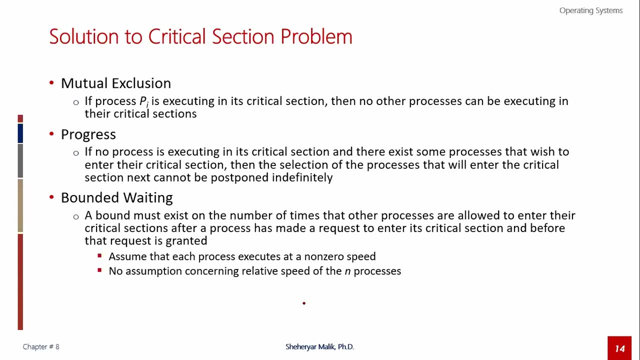 So if there are two processes which want to access one shared thing and want to access that, then one particular process will give one access to access that shared resource. So what are the solutions of critical section? Number one, and very important, is what we have discussed. 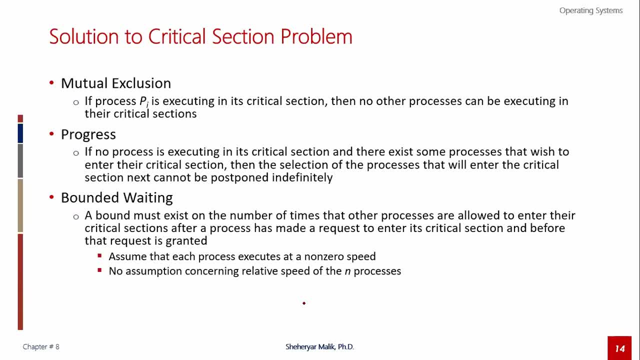 mutual exclusion. If one process is being executed in critical section, then no other process will be executed in critical section for the same resource. Remember this because these days we are having multi core architectures, multi process architectures. So if there are two different independent resources, 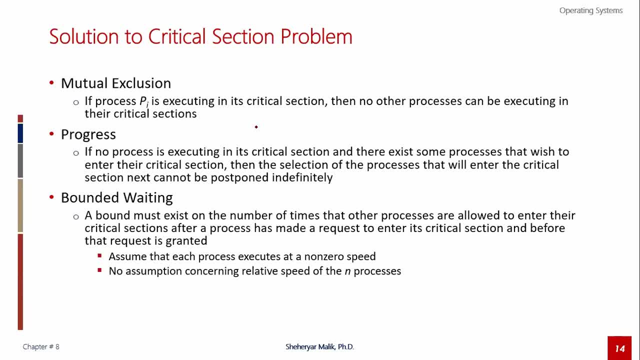 to access, then that is fine. but for the same resource they cannot be in their critical section, So you have accessed only one of them. Second Progress: if no process is executing into its critical section or any other process which is being executed in critical section. 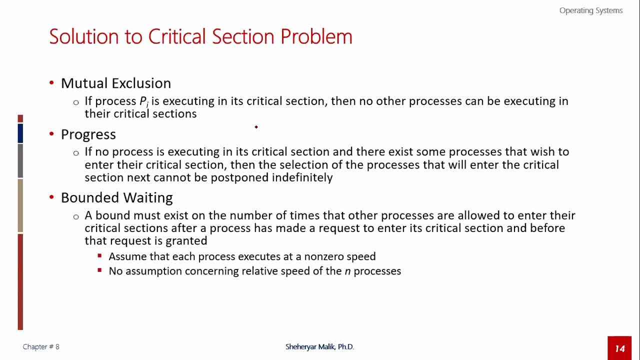 should not be in the waiting state. It should not wait. Similarly, bounded waiting should be done. A bound must exist on the number of times that other process are allowed to enter critical section after a process has made a request. So other processes are getting access again and again. 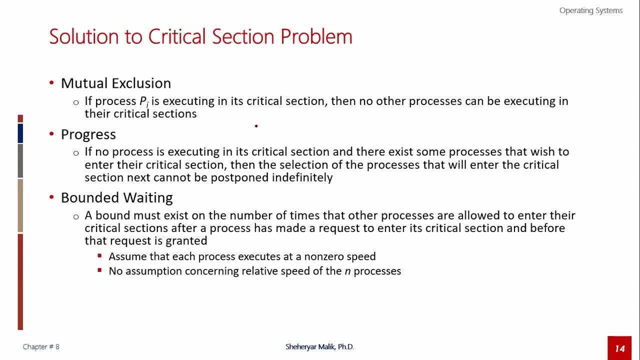 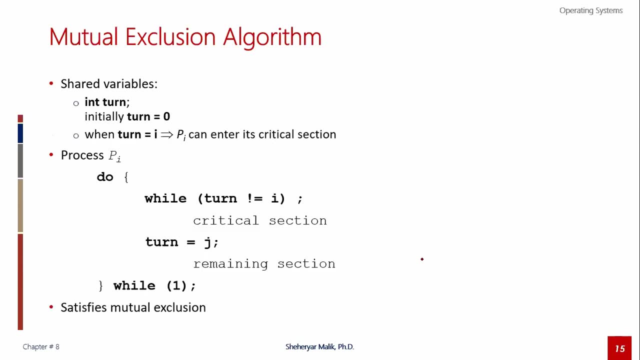 when a process is being waited in critical section, then it should not be that a process is waiting in the waiting state, So there needs to be a limit. So this is a solution for mutual critical section. So if you want to make a mutual exclusion algorithm, 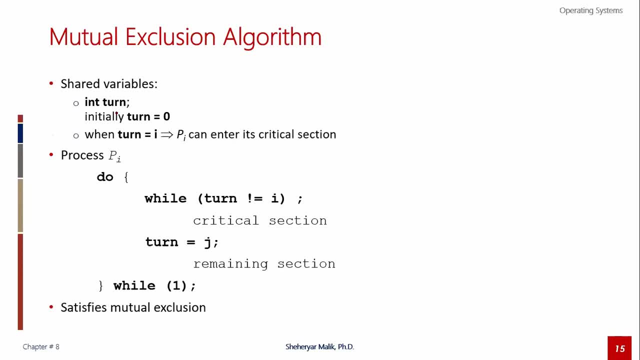 then what is its method? Let's say you have a shape, variable Turn. Initially turn equals to zero and one turn equals to IP. I can enter its critical section. So when IP comes, then process, I can enter. So what the process I is going to do? 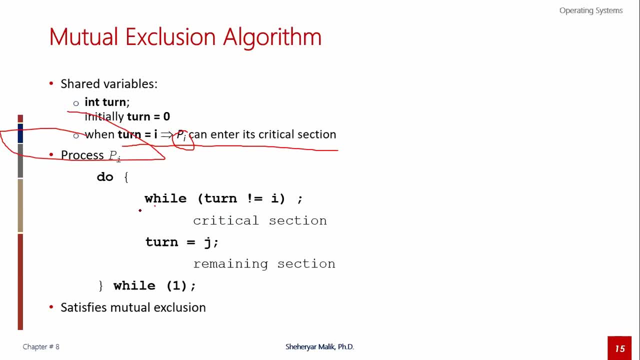 What will process? I do. It will enter until process. I is not entered. So he is doing what? here He is doing wait. So this is a wait state. Here it is waiting. It is waiting Once the wait is over. 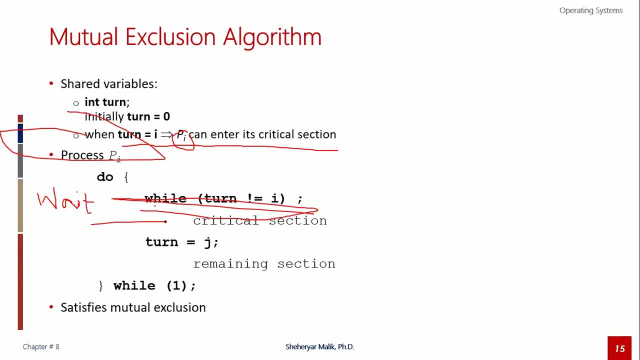 and turn equals to I, then what will happen in case of I? Now it can access the resource. Where will it access the resource? In its critical region or critical section? It will access the critical section. After accessing, what will it do? 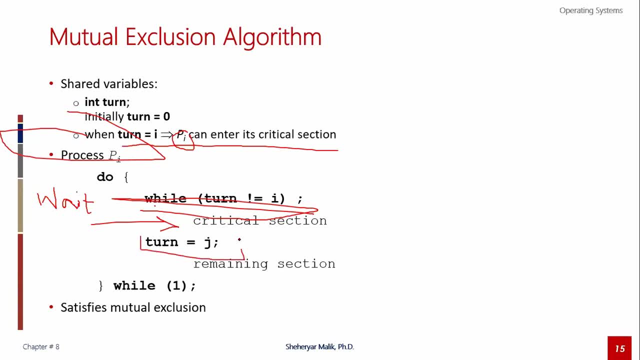 In the end, it will come out of this critical section And what will it do to turn? It will turn to next, Which is J, And then it will execute its remaining section. Here you can see that the rest of its code is different. 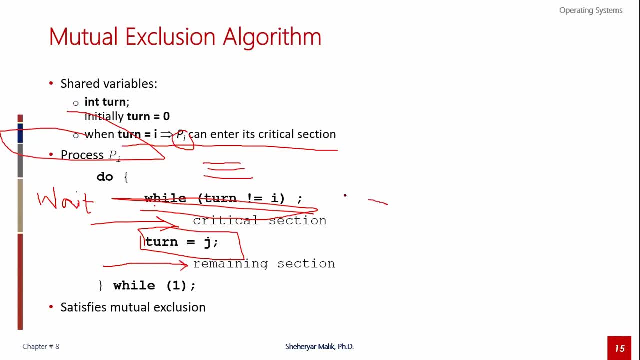 Here before this there is another code. This is the area of critical section. This is whole critical section related stuff. In between there is a critical section and in critical section the entry is not direct. Before that it is waiting. What is it doing in wait? 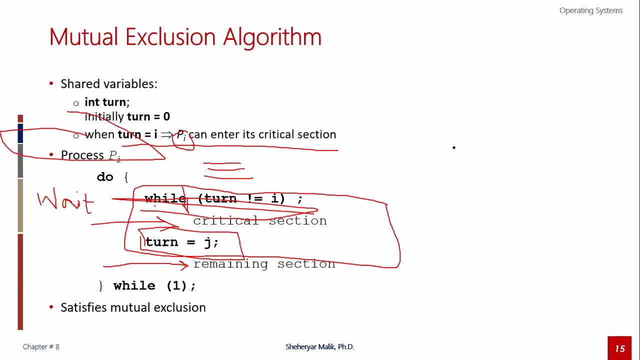 It is checking in wait that whether the turn will come or not. The J process will keep checking whether the turn will come or not. If its turn comes, then it will be able to enter the critical section, Otherwise it will not. And once it is exiting. 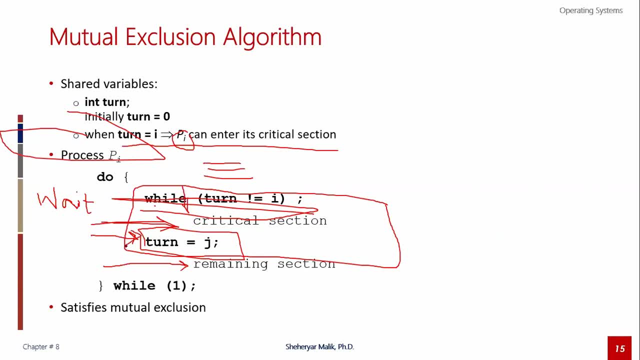 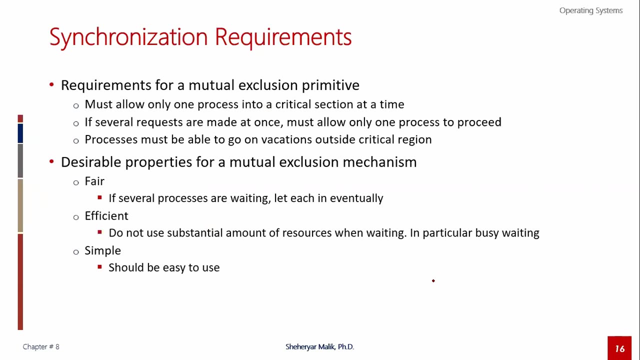 it will change the turn to the J, It can use the next turn And then it will execute the remaining section. In this way, your mutual exclusion is implemented. In general, what is the requirement of synchronization If you want to have a mutual exclusion? 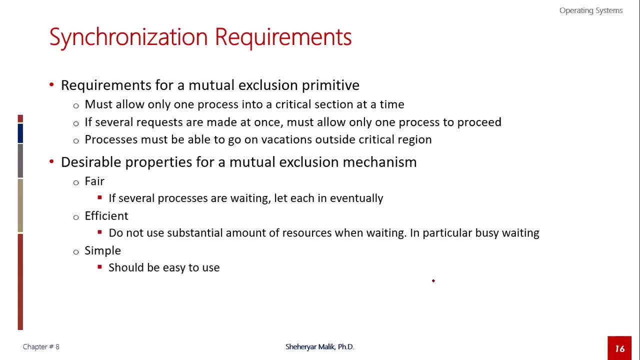 primitive. the main characteristic of mutual exclusion is that only one process can execute or access the shared resource, Means only one process can enter into its critical section at one time. You cannot have two processes. If there are multiple requests, you have to only allow. 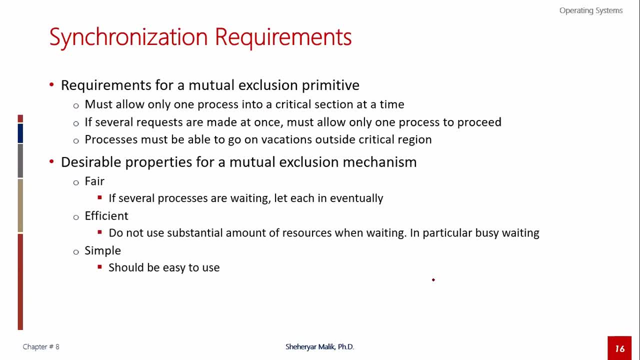 one process And when it comes out of the critical section, it should be able to execute the other process. It is not relevant to this shared resource. And what are the desirable properties? Number one: fair. It should not be biased for some processes. 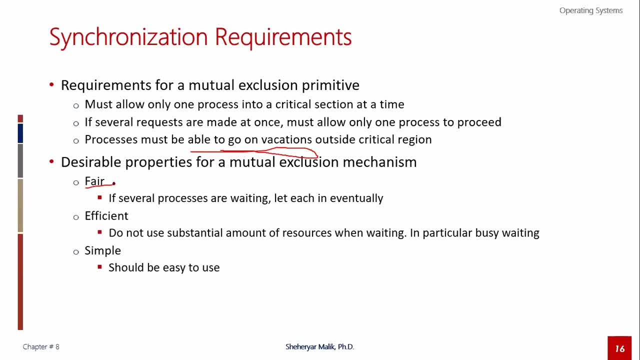 It should be able to give access to multiple processes. It should be able to give access to multiple processes. Number two: efficient. There should not be too much time in waiting for the resources. And what is a major way to do that? Every resource, every process. 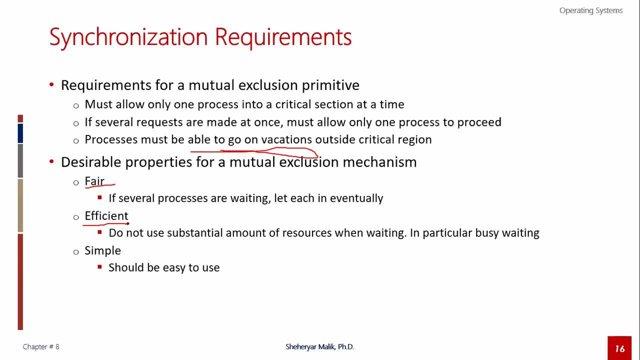 wherever the critical section is made, it should be able to access the shared resource. The critical section should be very minimal, Only to the point, Only that code or that thing where the shared resource is accessed. When every process will do this, it will automatically. 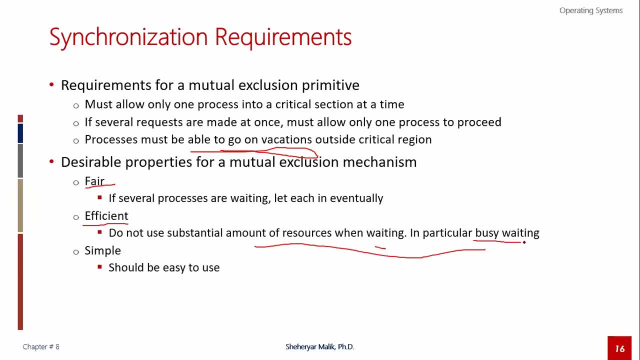 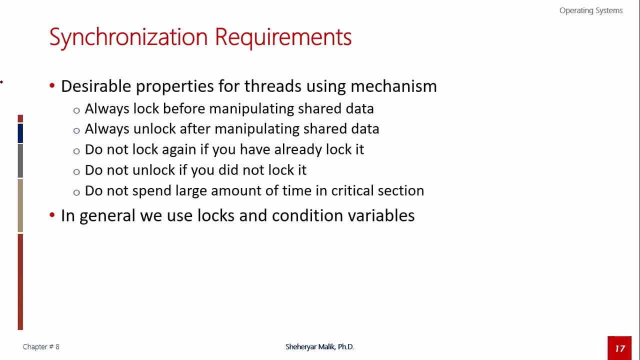 be reduced So they will not waste their time in waiting. And number three, simple. The mechanism should be very easy to use. This is very important. So what are the requirements for synchronization? Very important When you want to do mutual exclusion. 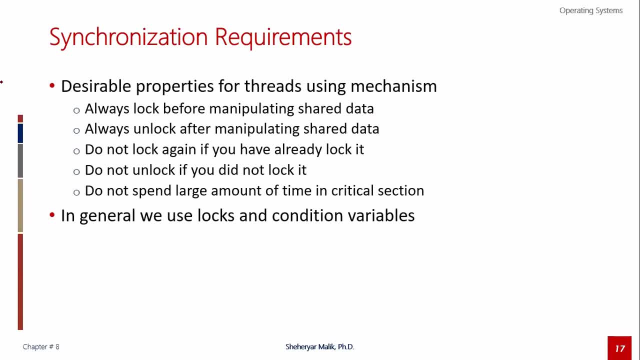 when you want to apply critical section. what are the requirements for synchronization Thread process task? you will have to apply it. Number one, what is the most important? You have to lock the resource. Whatever shared data you have to access. 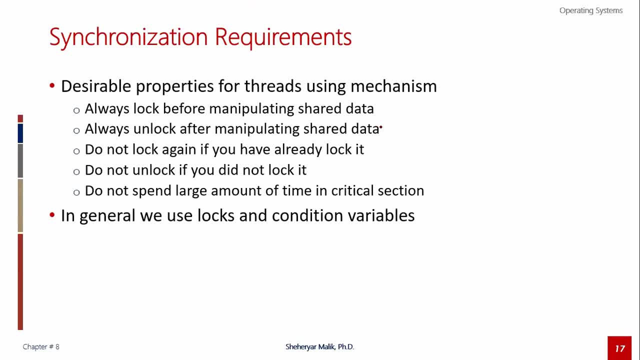 you have to lock it first. This is the waiting mechanism. What does waiting do? It keeps waiting. Whatever is its turn, the first thing it does is to lock it, And whenever it is finished with its critical section. if it does not unlock, 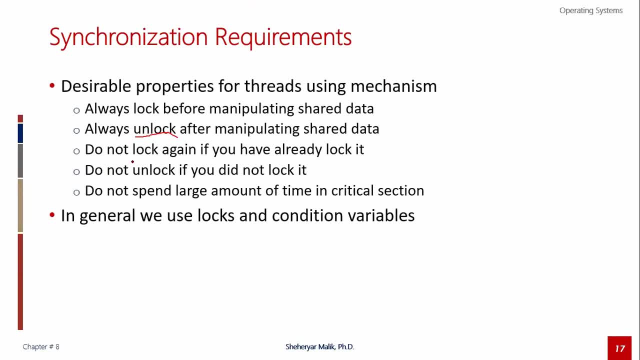 the rest will be locked In the same way. do not lock again if you have already locked it. In the next lecture we will see some synchronization mechanism in which there are semaphores and monitors, So you will have a better understanding what happens if you lock again. 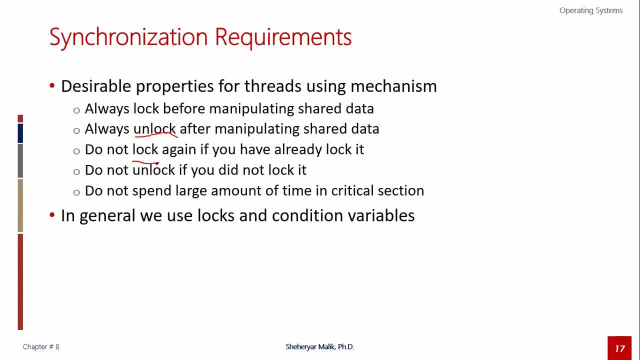 because they use variables for that, So that can be a problem. So if you have locked it, do not lock it again. Similarly, if you have already unlocked it, do not lock again. And, very important is, do not spend large amount of data. 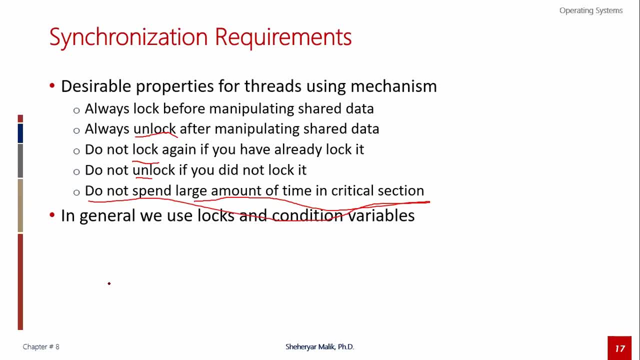 sorry amount of time in critical section. Critical section should be small. This is very, very important. Spend more time. Why, If you spend more time, then the rest will be locked. Rest will be locked, So they are going to spend. 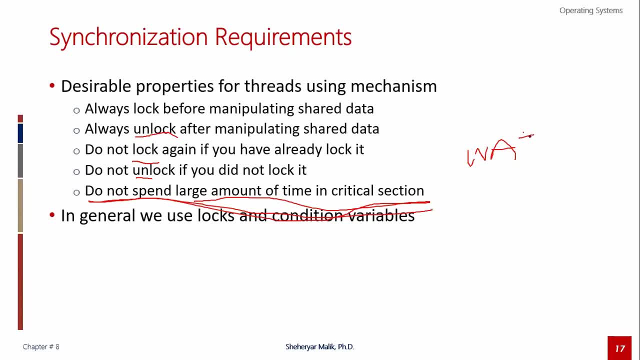 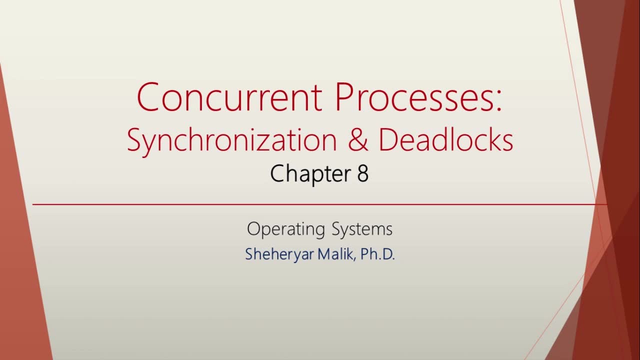 a lot of time in waiting state. So it will be in waiting. And what happens in wait? It is wasted. So generally we use locks for that, which we will study next lecture. That's all for the topic of concurrent processes And thank you for watching.